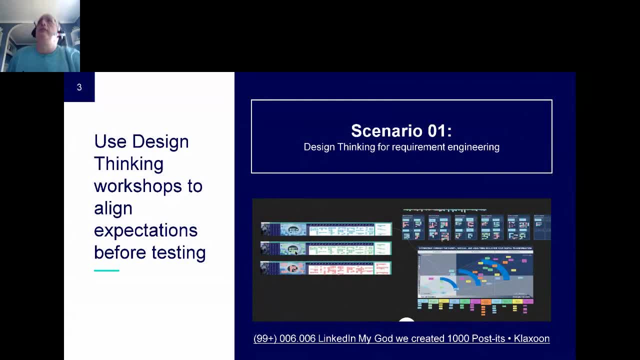 And the second scenario is about using design thinking for testers. And the third scenario is about using design thinking for actually building your team experience. Now I'll give you a short example how that would look like if you're actually doing a workshop to gather those requirements and not jump into a click zone. 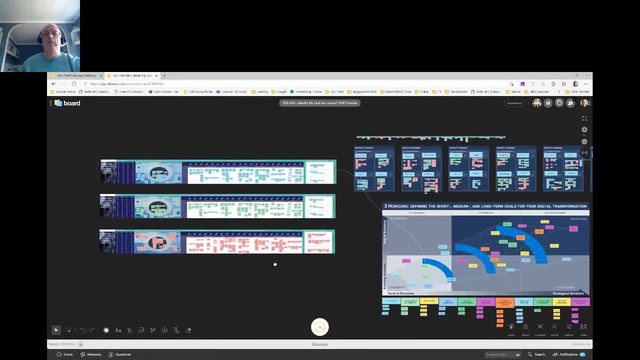 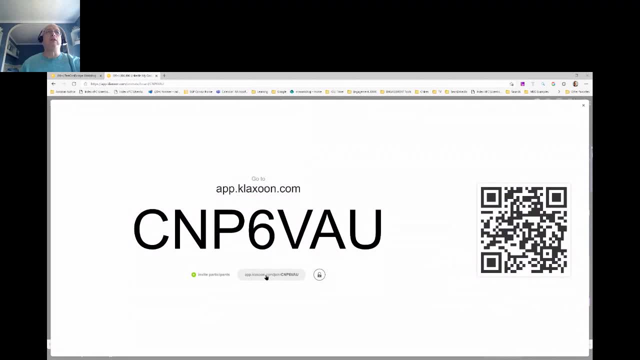 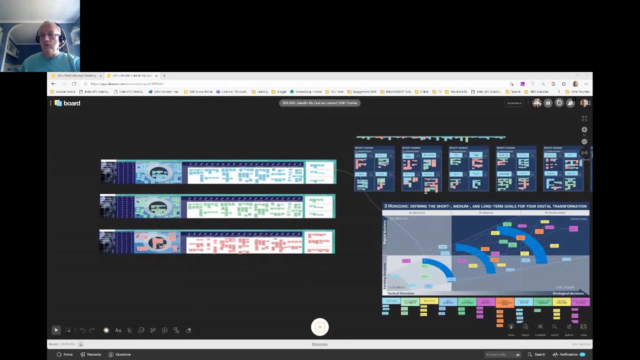 Also share this so you can have a deep look at this later on. So I'll just put the click zone link into the chat And you can then join and also explore this um, this example. so here's the link for you. so the basic idea about all of those workshops- how do they work- is you create a poster in. 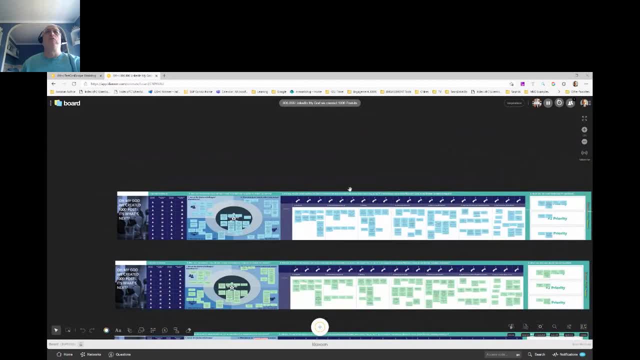 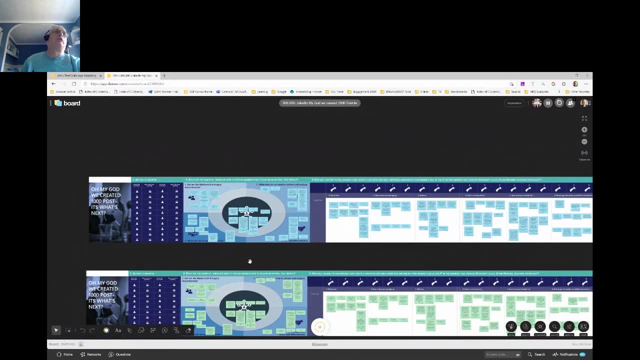 clickzone and you have an uh a topic. this is from a linkedin article, so all of those uh posted to erc uh are kind of fabricated- it's workshop because i can't share it. but in general you can have a topic that you want to work on. then you're going to have um a section where 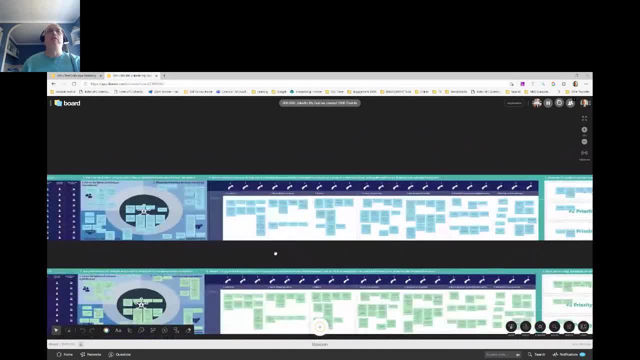 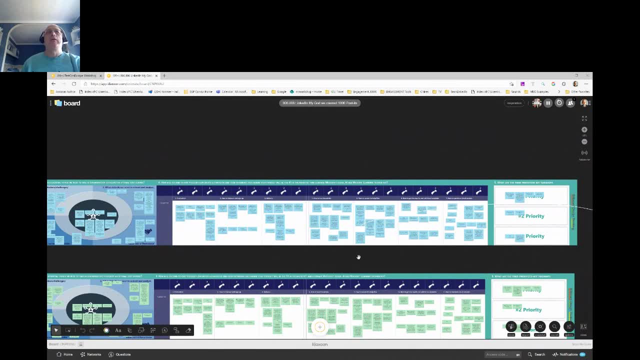 you can look for new ideas and in many cases you're going to build, building your application, a user journey or the product that you actually want to work on. and now the nice thing is you're collecting those requirements in a workshop and you kind of look into those detailed ideas. 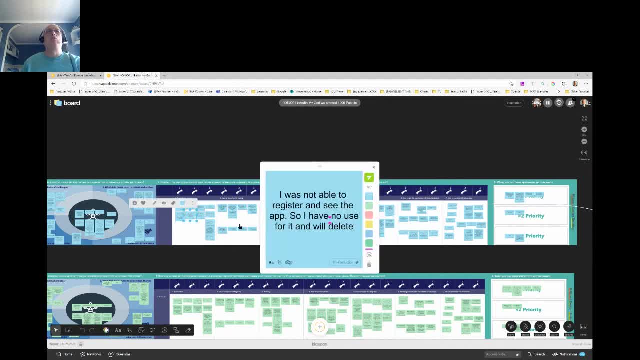 this is where actually the link is to creating those user cases, those use cases and you directly can convert them actually into test cases. like i was not able to register and see the app, so i have no use for it and i will delete it. and that means now you can kind of create those user stories and 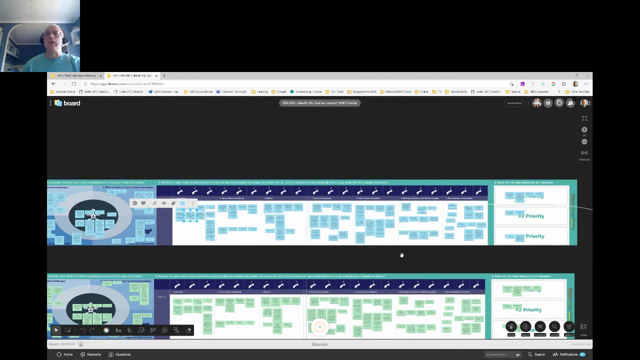 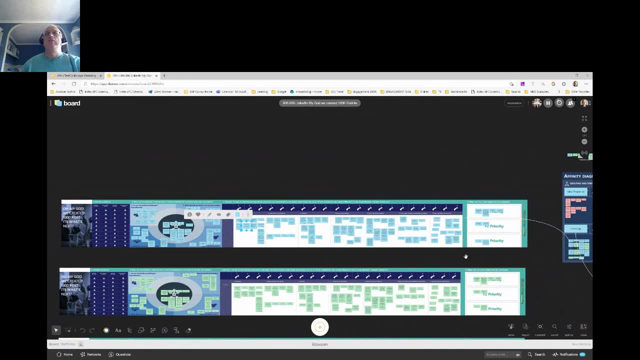 with the end users together and then, in many cases, um, from those user stories in general, what you're going to be doing when you're creating those requirements you're going to be looking for is, uh, for example, if you're using an affinity diagram, you're going to be looking for the 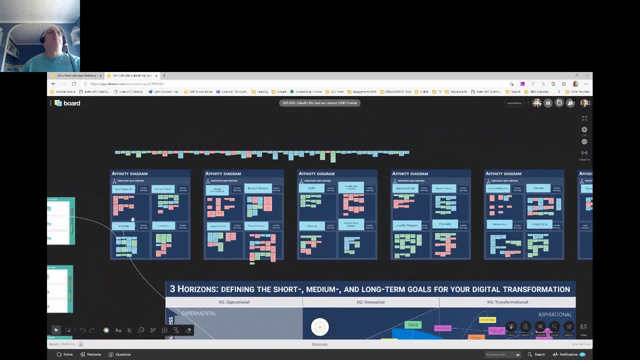 user stories. and so what we're going to do is we're going to look at those different user stories and then kind of look at the different uh applications and then the different requirements you're crafting. your solution is you're going to go into a second step and this: 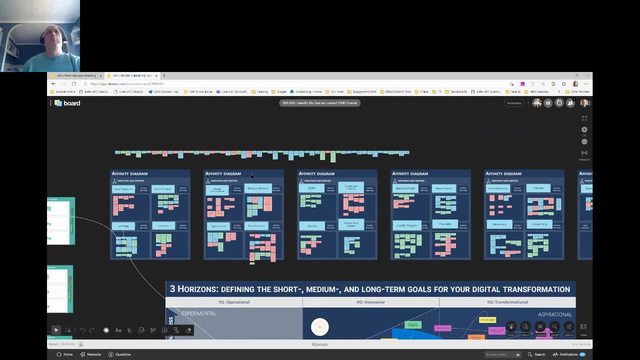 is more, let's say, uh, typically using affinity diagram, and what that means is you're going to look at all of those individual user stories and try to find out, let's say, synergies or topics, that a good way to do it is to put all of this into a three horizon map. and what you're actually doing 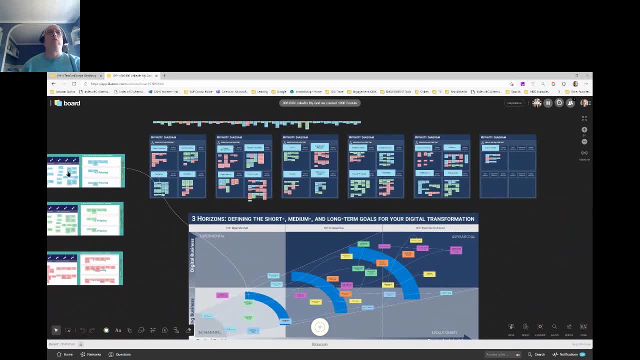 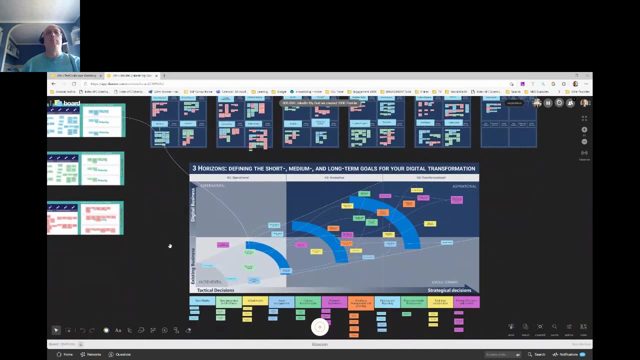 is you're taking an abstract end user requirement, like i want to get it. the security of my app is not going to expose private data. you're finding basically a topic where this fits and then you're putting this into a technology roadmap. so this is a typical way how you can um use design and 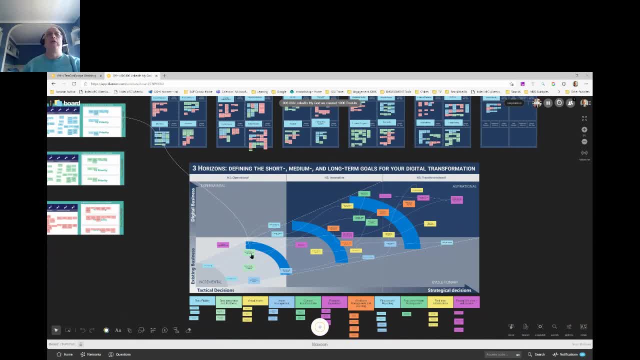 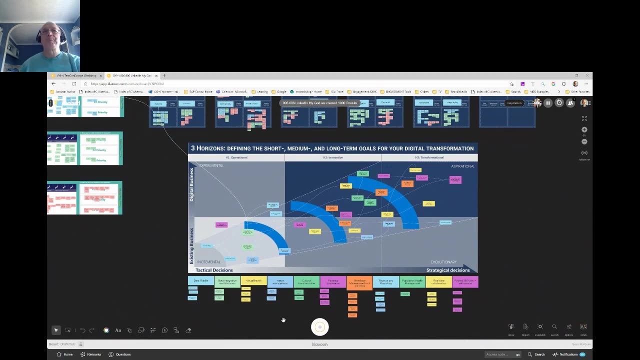 engineering and linking those to real use cases. so the nice thing is, once you create this technical roadmap or the technical solution, so you see, for example, here in the bottom, things like data fluidity, data integration, asset management and things like that- now what you can do is you can always link. 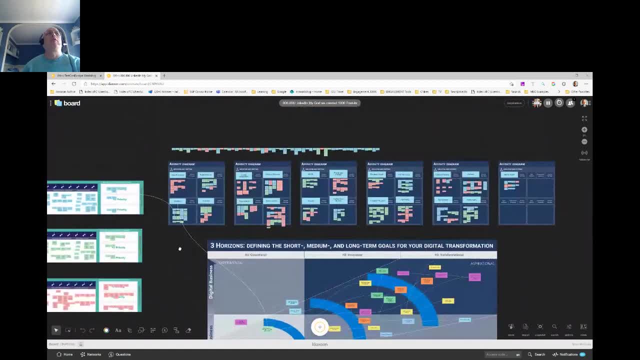 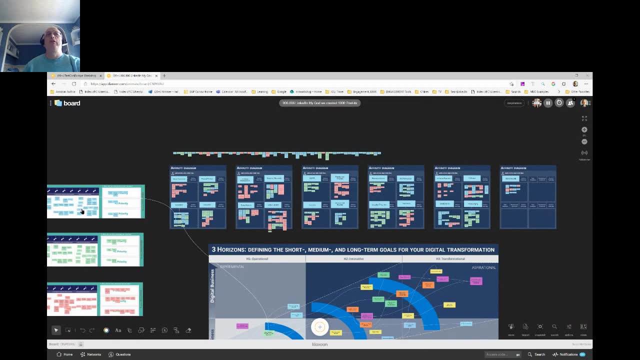 those technology bits over the affinity diagram, to what are those requirements that actually created this, and then you can look back into the conversation, into the workshop. why is that helpful? because, in the end, when you're uh trying to build your application, you always want to be sure that, uh, by creating the solution, 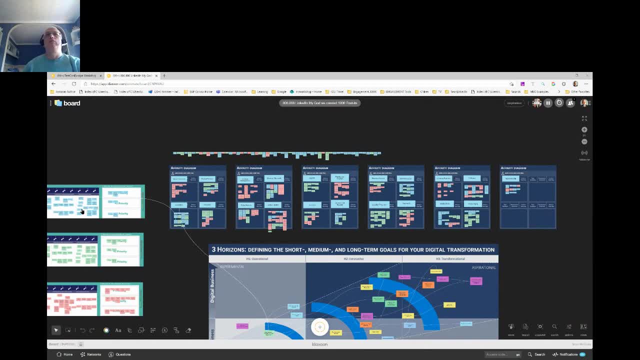 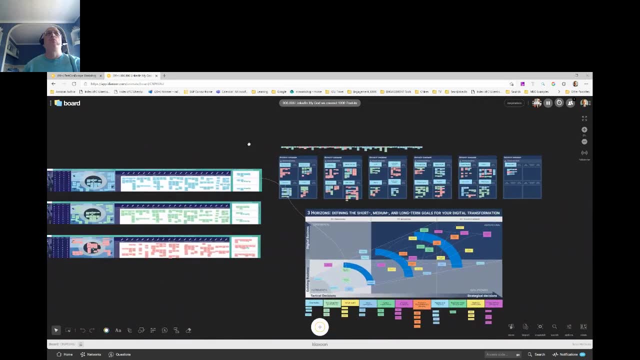 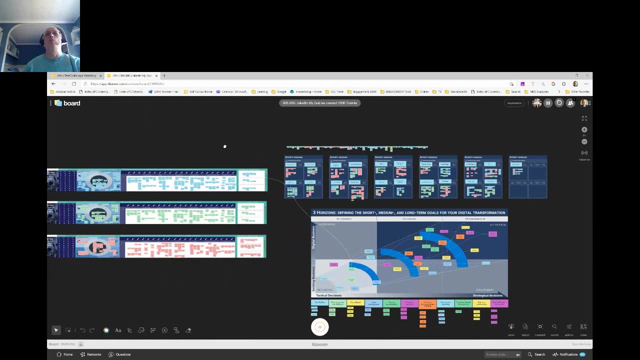 the technical solution, you don't use their perspective of the end user. so i'll come back to this later idea, how this actually technically works. and, uh, what we're going to be talking about in in the session today is how you can actually craft, uh, this design thinking workshop to have. 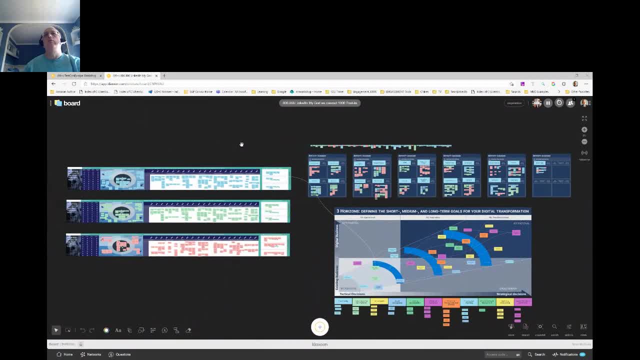 a better understanding of what's going on in the design thinking workshop and how you can actually have a better alignment with the customer and when you're crafting the solutions in the beginning and also use them for the testing. so, going back to the powerpoint, that was the first scenario where i would see that design thinking workshops can help you. 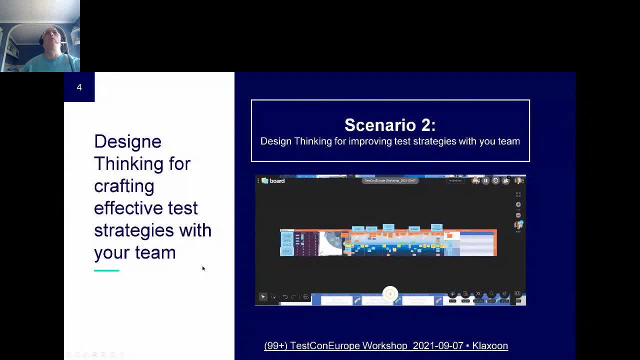 and i shared the link so you can go there afterwards and explore it. the second scenario that is very interesting is you can use design thinking workshops for improving your test scenarios or i actually creating a test strategy. i had a workshop two days ago. it was a full workshop, part of the 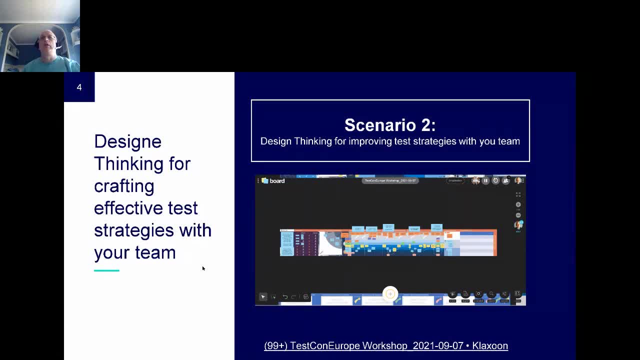 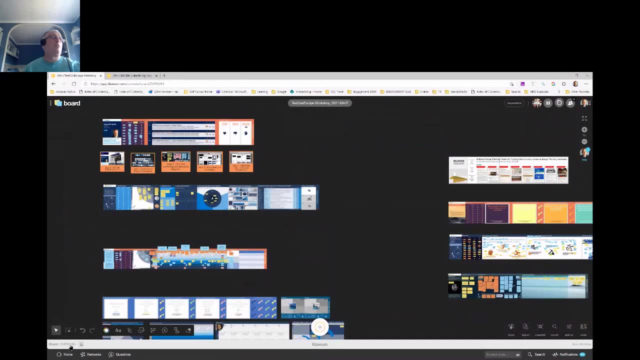 conference, we were working on the same topic, and what i'll share with you is an example: how you can, uh, build a workshop. that's really about your testing team and your testing abilities. so what i'll show you here- the results of this, and again, i'll also share this, so feel free to explore this. 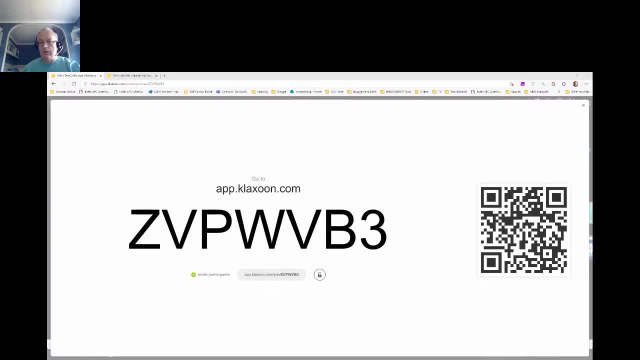 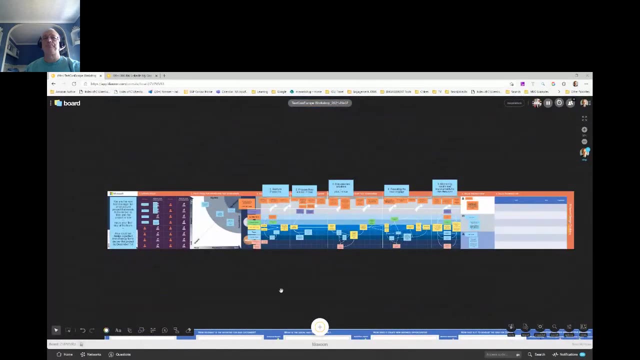 and go into this. uh, see how it goes in the next slide, please. those details look like And here's the link. So what we did here in a brief session and it was just part of the training that we had two days ago And the question was like what would be? 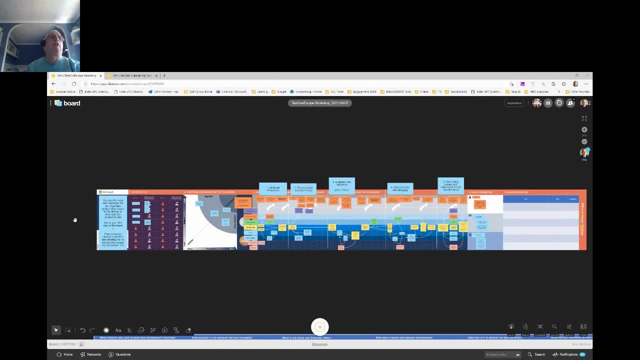 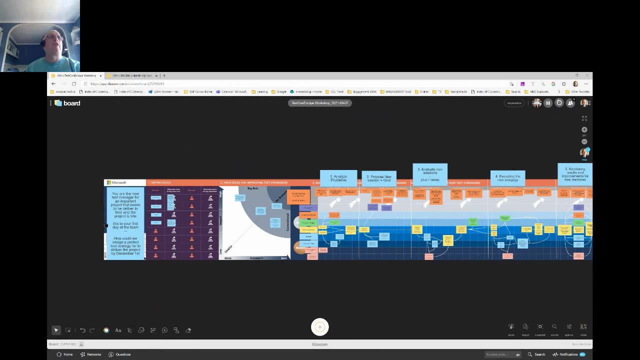 interesting from a test perspective, And here we had, let's say, as a topic: you are a new test manager for an important project that needs to be delivered in time and the project is late. This is your first day on the team. How could we design a perfect test strategy for delivering the project? 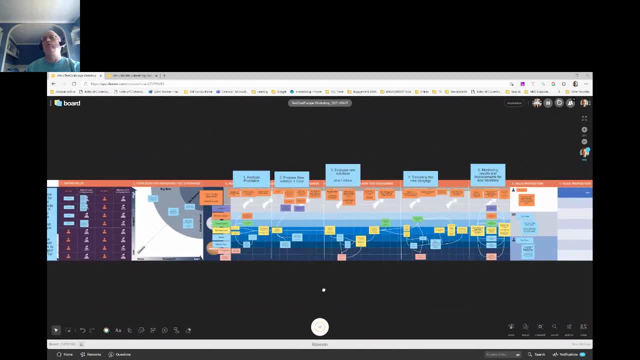 by the end of December, So it might be during a project. you have to deliver your testing application or all the tests within a specific time frame. Typical things that you might have is, let's say, budget time restrictions. Maybe you don't have enough developers to help you with the. 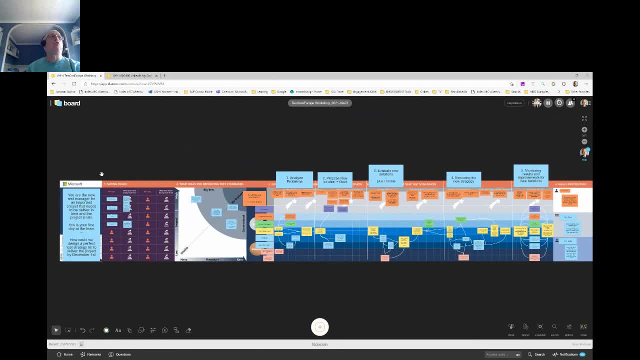 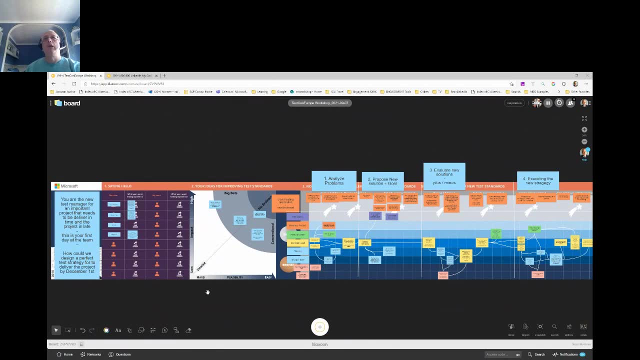 testing. It could be almost a year And you have to deliver the test within a specific time frame. It could be almost everything. The way this workshop was structured was just saying hello is a typical way, just so you know who's participating. You can do these workshops physically in a room. 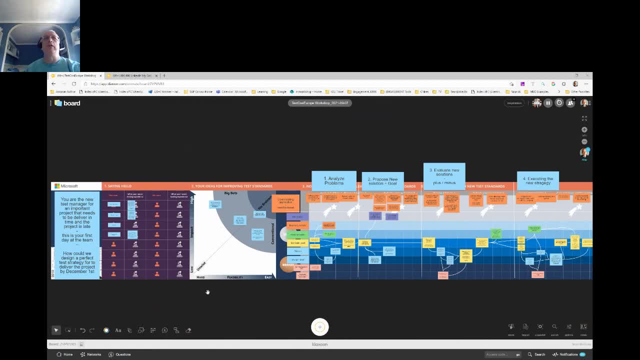 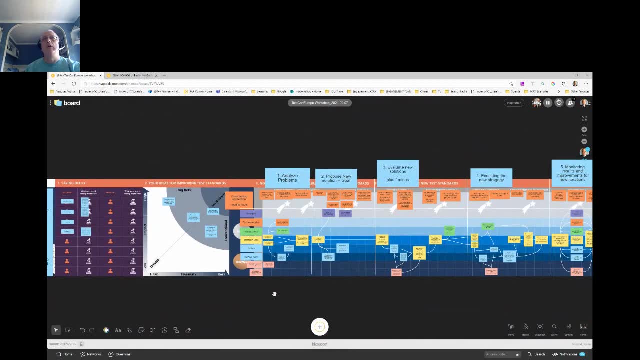 where you just print out a post or you can do them online, as you see here in Klaxon. Then the first question is: what general ideas would you have for improving those test standards? So imagine you have a smaller or larger team- Maybe it's five people, Maybe it's 20 or 30 people- And you're 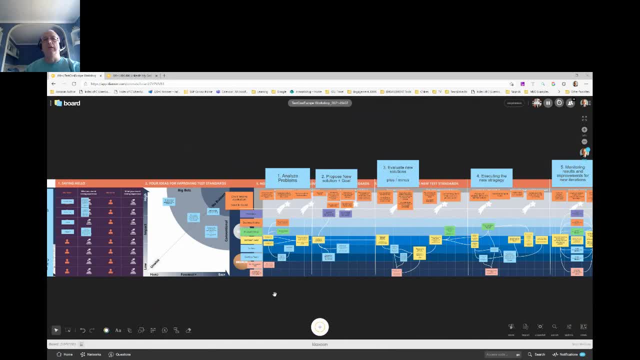 trying to build this test strategy And you have to deliver the test application And you have to deliver the test strategy. And design thinking basically says: well, first try to explore the problem space you have. Invite those people, Have the conversation And they will typically be. 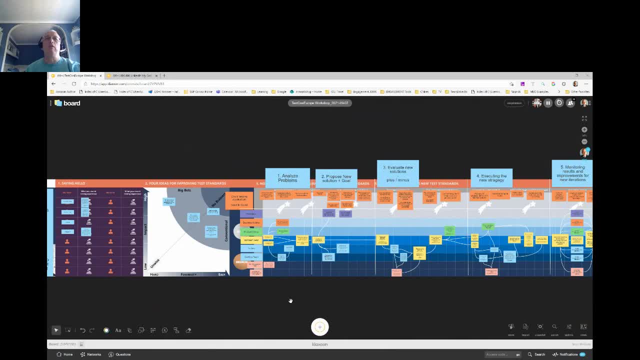 sharing things within your organization Like: oh, testing is confusing because people are sending updates with emails And then we don't know what is the last status. Or, if we test, it just takes long until we get access to the test environment And then we have to use dummy data. 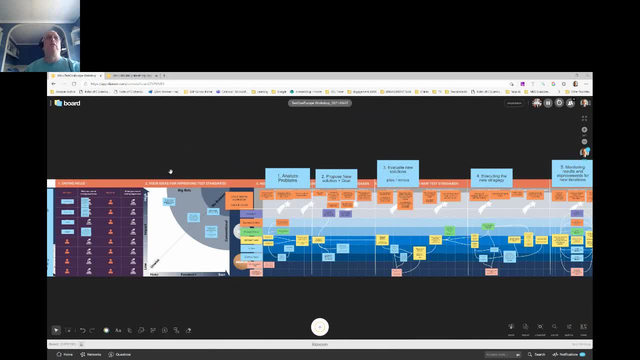 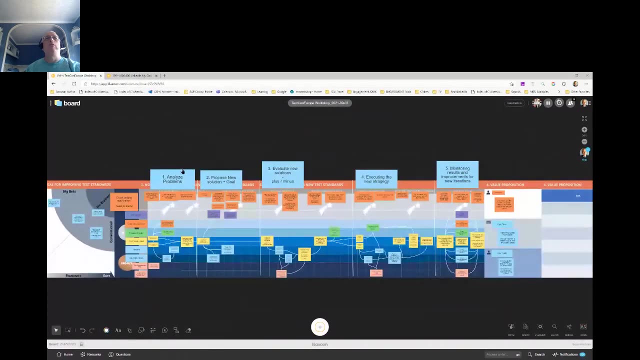 But with the dummy data we can't actually do the real tests. So this is like a typical way that you kind of first select information about the current state And here there was like basically, let's say, a voting- What are those top three? And then you see this is a little bit messy, But this is also. 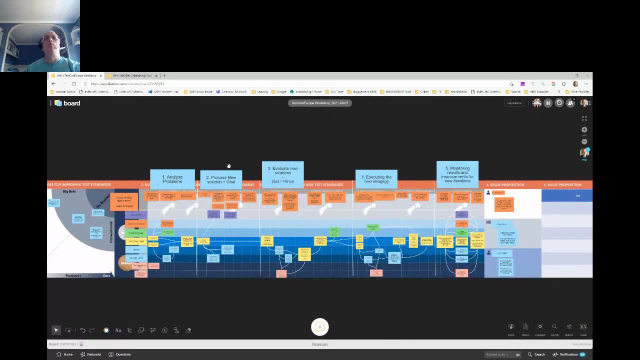 kind of typical for design thinking that you go into a workshop with the assumption how you want to build something, But actually having the conversation with the experts it turns out that things are very different. And the way we kind of split this up was: first you would kind of analyze the problem. So if you're assigned to the 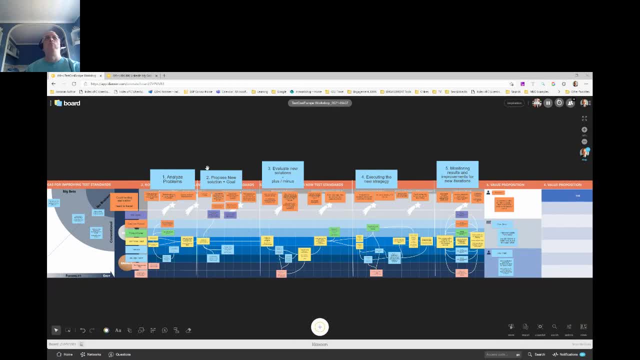 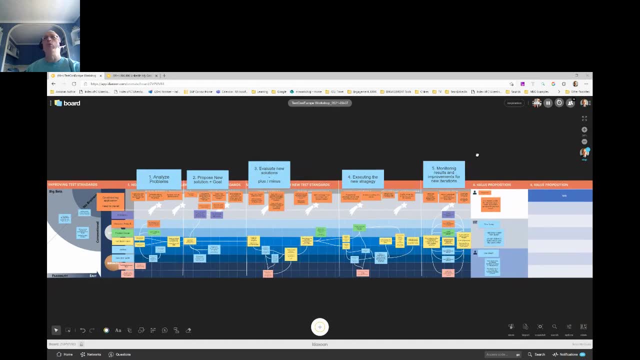 test team. you need to manage this test team. Then you would actually propose some new goals, You would evaluate the solutions, You would then execute the strategy And then, of course, you would be monitoring results, improvements, with no iterations. And here we had basically like swim lanes, We have the manager. 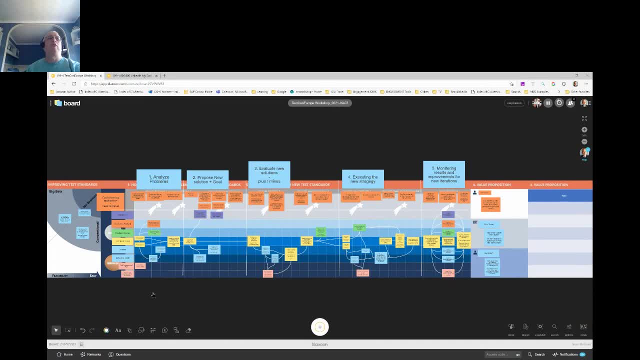 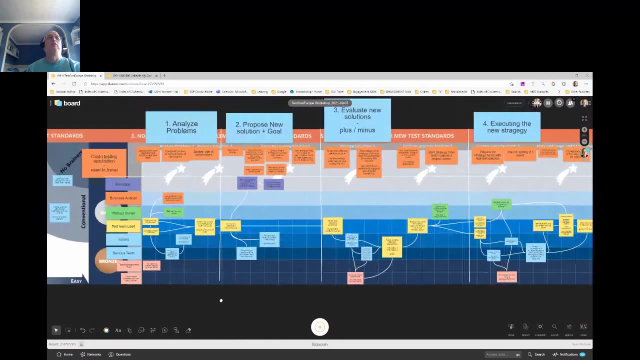 business analyst, product owner, test team leader, tester and test developer, And the idea was that was the first part. Who is actually involved in this complete end to end testing process? And, without going through the details, we can go and explore it on your own. What is the? 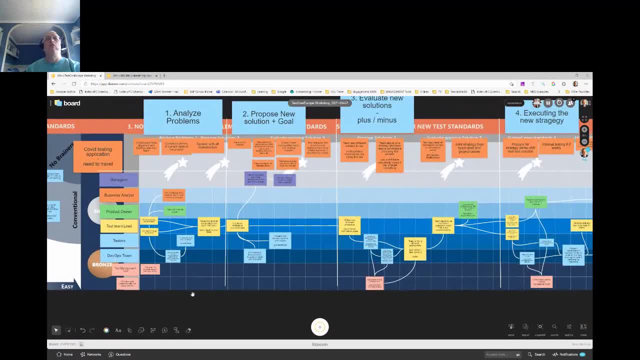 idea of this kind of a workshop is: Are you going to have a conversation with the people that are involved in your team, that are relevant And, let's say, for test team lead? he will first check the roadmap and the deliveries. He will also kind of use the statistics about the bugs they had in the 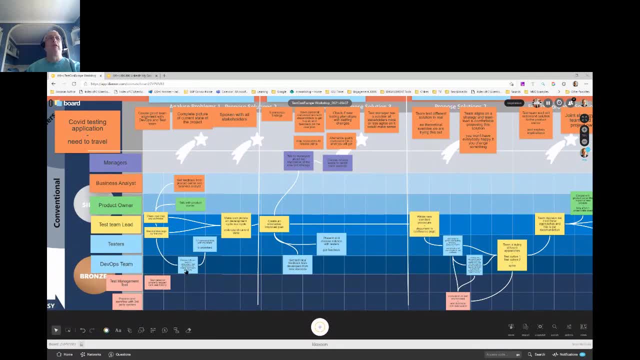 past and he'll probably sit down with the DevOps team to discuss like: what are their preferences? how would they want to test? he's also going to have a conversation- a one-to-one conversations- with the testers. at the same time, he will need to have some conversation with the product owner. 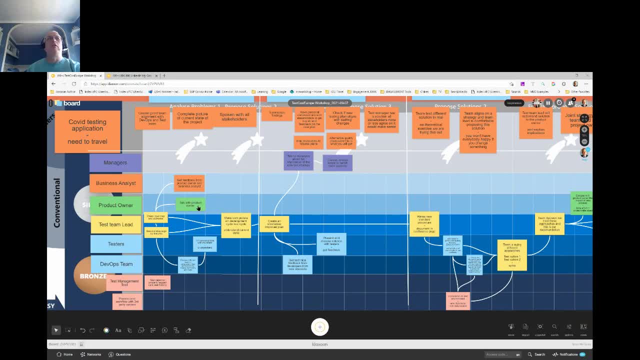 because maybe test strategy could be to test different stuff or less stuff, or improve or reduce regression testing. so there are many strategies and it might just affect the end product that you're delivering and then also getting involving the business analyst to kind of think really about what's important. what you just see here is that you kind of use this. 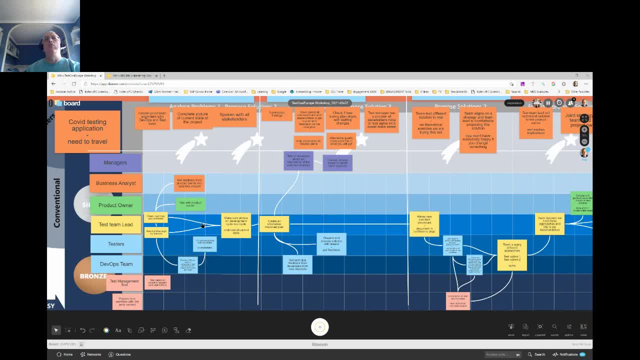 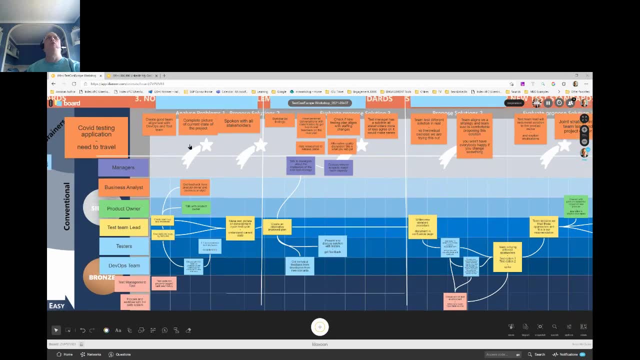 workshop and this will usually take maybe two or three hours to capture those ideas and in craft a new solution how you want to do those testing stuff. hope you just have the high level things you're doing for each step, like create good team, align with DevOps and testing. complete picture of. 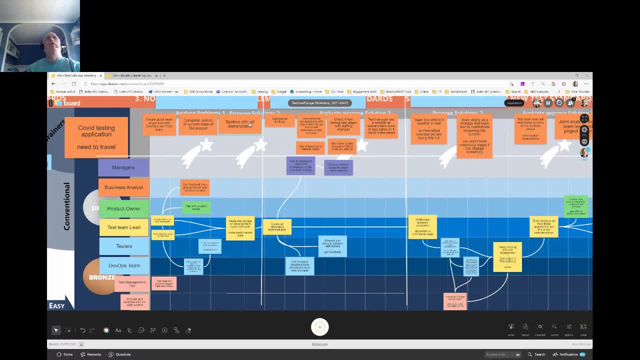 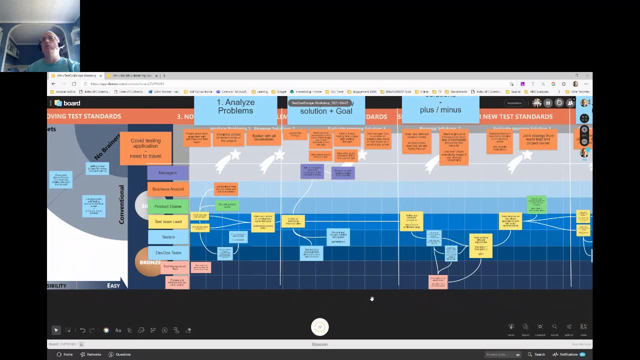 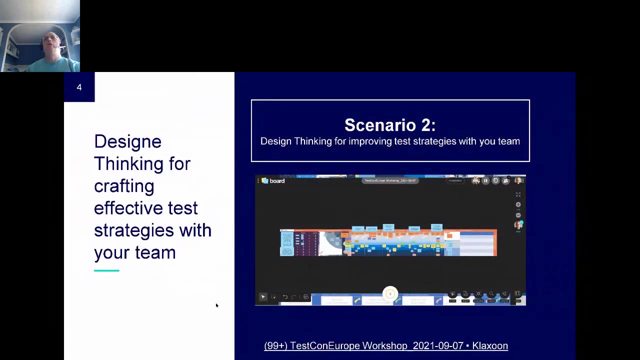 current state of the project and you spoke with all the stakeholders before you actually went into crafting a new solution. so this is typically what you can do, how design thinking could actually help in this, in these scenarios. going back to the presentation, what I would want to walk you. 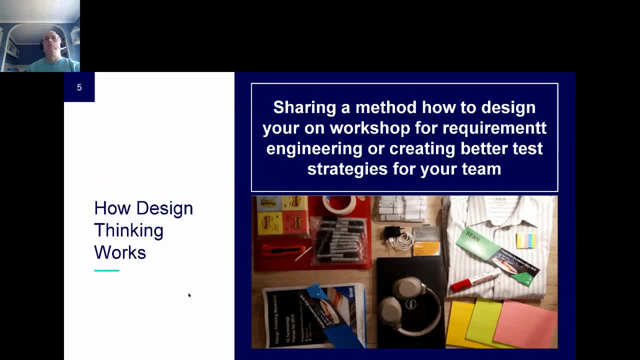 through is, let's say, a simple way to use this method to build both either the workshop for you users, for your customers, in terms of requirement engineering, creating those use cases, as well as, basically, let's say more to change management aspect. how can you use those for team building? 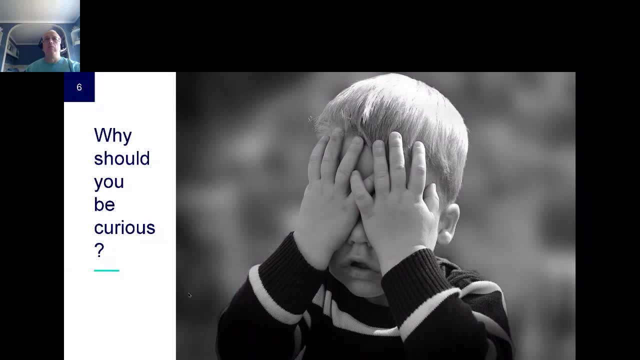 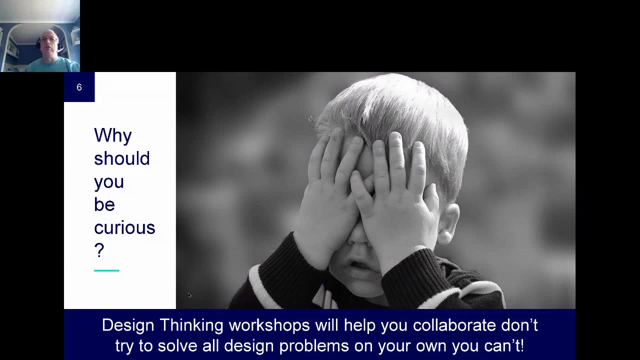 internally. and the first question is: why should they actually put design thinking on, let's say, on your agenda, or why should it be interesting for you in general? and I really believe in the end, in order to be successful in anything, especially in the software business is all about collaboration, so really think about design thinking. it's a 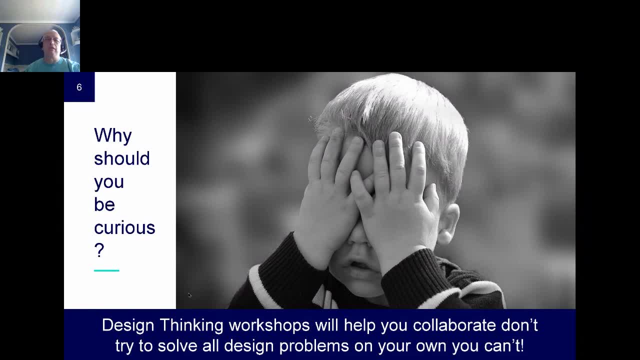 collaboration tool. good collaborators are successful and if we look into the software project, if things don't work, it's always about collaboration. it's about misalignment, people misunderstanding things, customers thinking to getting something that they won't get, or software developers thinking you need to develop something that's not in scope and 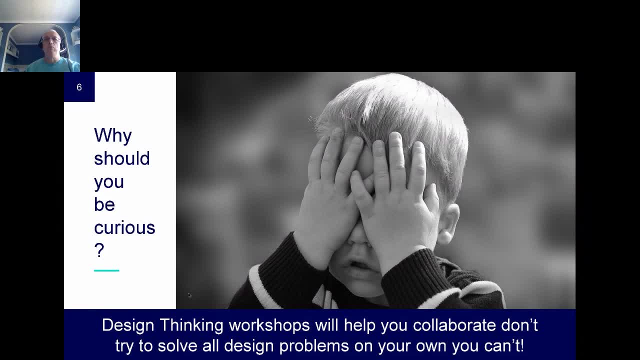 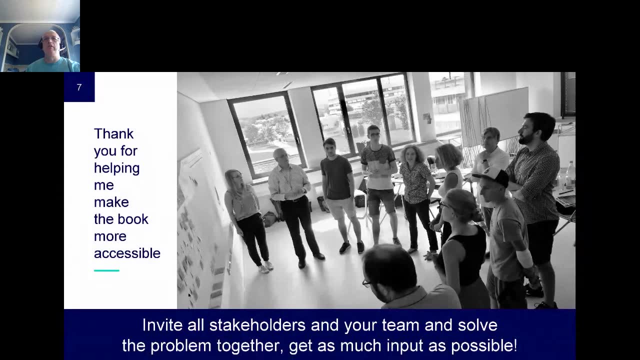 things like that. so really think of design. thinking is a collaboration tool. how are you going to do it, no matter what problem you have? if you're building an application, if you're discussing with your customers, or if you're building a test strategy or trying to improve your 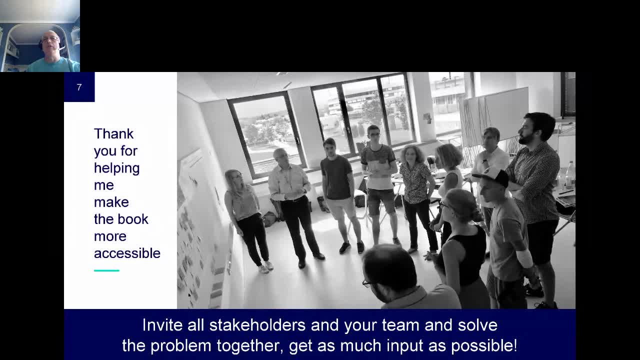 test cycle. it's very simple. it's just find people that care about the problem, get them in a room and have a conversation, and design thinking is all about listening. you always have your own opinion, and what's going to change your opinion, what's going to improve it in the end, is really about 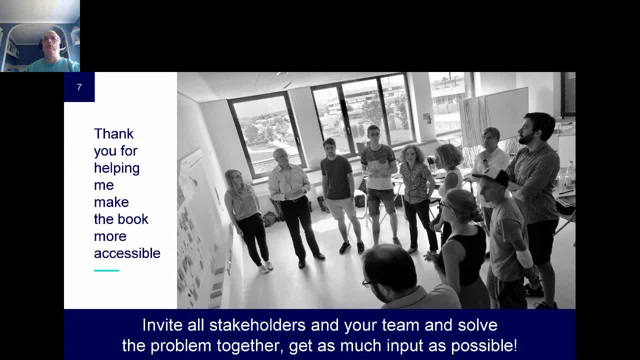 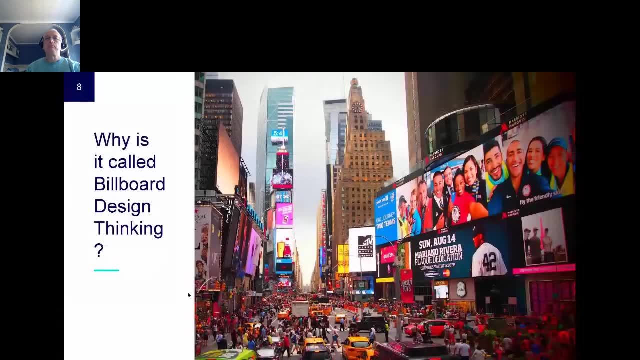 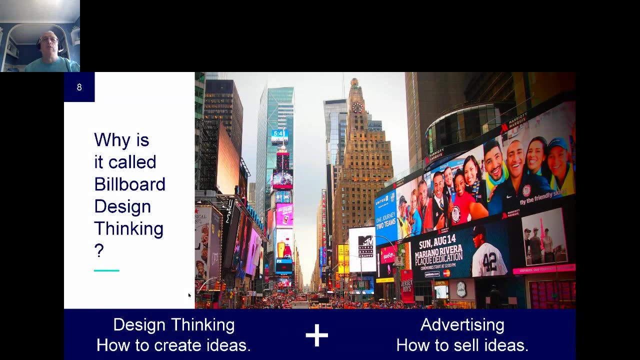 input from other people, and design thinking really is a tool to get other people involved. if you lean back and listen, that's basically the whole power of design thinking. now just one slide about why this is called billboard design thinking. what's the idea behind it? after being in this business, 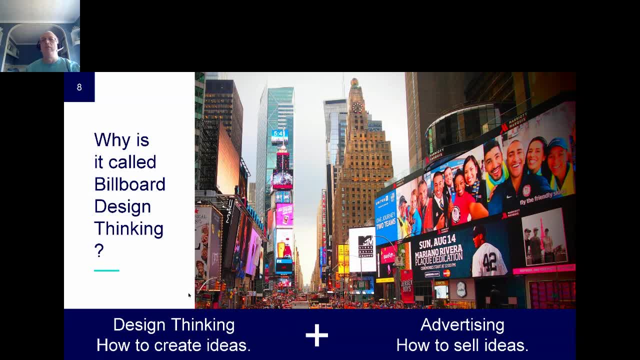 for many years and doing 500 plus design thinking workshops. the one thing that kind of frustrates you is you have all of this excitement in the workshop. everyone says, oh, we have this great ideas. this is the way we're going to change our process. this is the way we're going to build a product. but if you look back, maybe five or maybe. 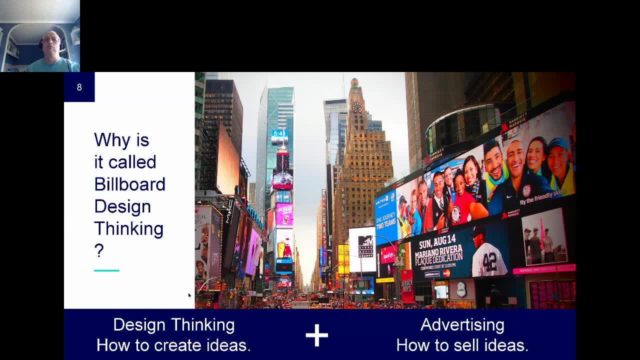 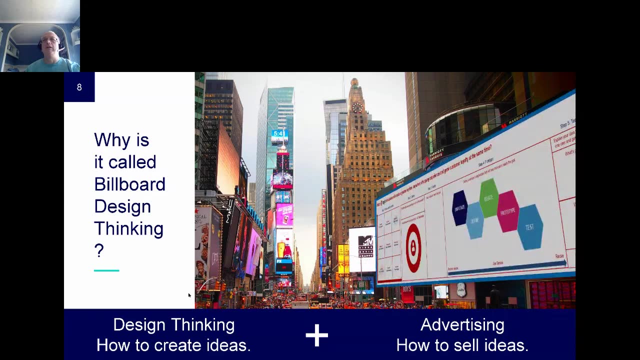 only two percent of those workshops really then create real change and make it to to the product. so what's the real problem? well, taking this excitement and all of those ideas is not enough. you actually have to sell it, and this is kind of the combination between design thinking and 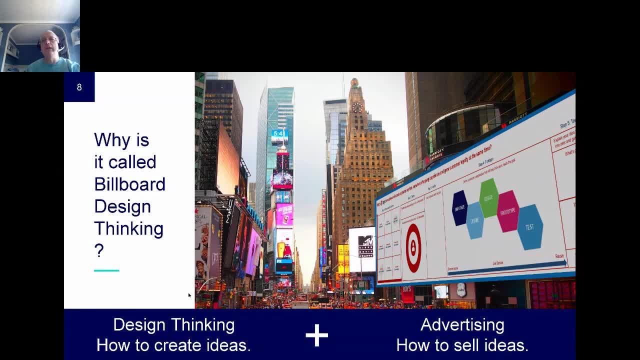 advertising used to design thinking to create those ideas and use the design thinking to create those ideas and use the design thinking to create those ideas and advertising actually to sell the ideas. um, and be very conscious of that, and as you will see later on, uh, you will always create a poster, and what's the compelling thing about the poster? poster. 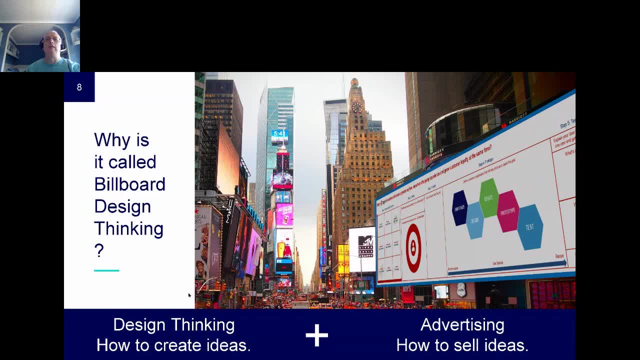 usually you will find next to a highway or a place where people have really little um or spending little time, have little attention. in the end, it always has three elements. the first thing: it's going to tell you what it's about. yeah, for example, you deserve the vacation. there's going to be an. 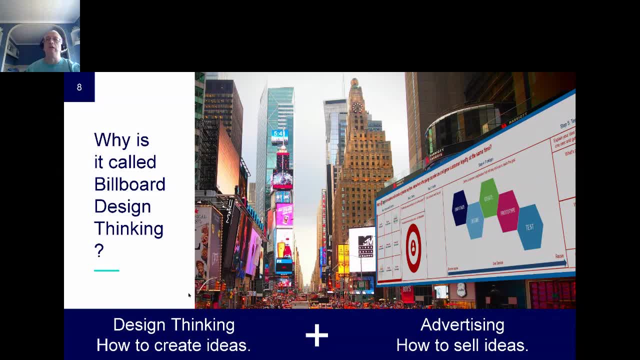 image. on it it's like a beach of highway, so maybe a place you want to go, and the bottom it's going to say, um, just 9.99. so it's always this combination of a clear agenda what you're talking about, a visual that's going to help you understand what the product is about that you should be buying. 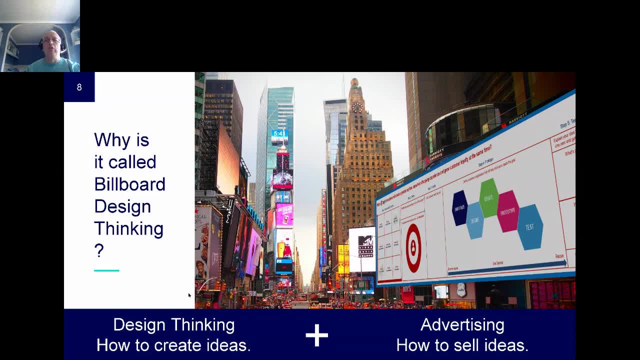 in a call to action. so if you combine those two things and you use your design thinking workshop to create the poster that you're going to use to sell your idea afterwards, internally, to managers, to customers, to partners, to product owners, that's the real power and idea of using design thinking. 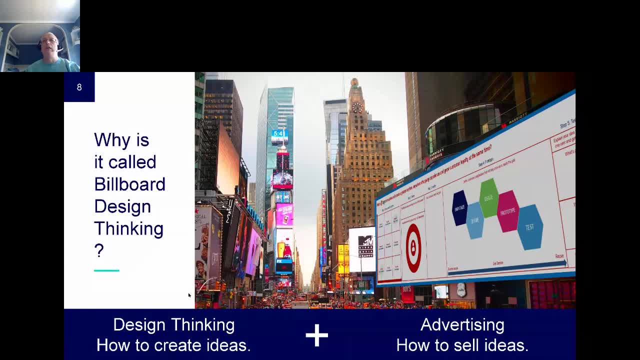 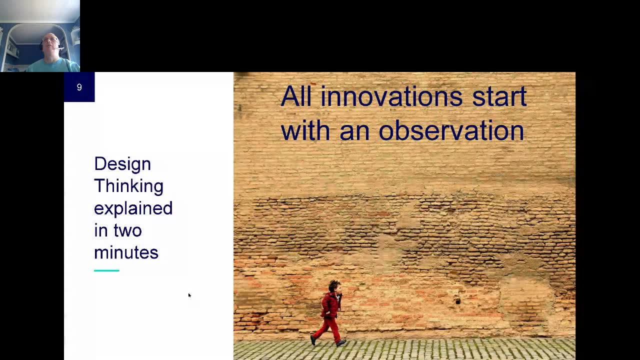 in this sphere. so just three slides about to get everyone on the same uh level or understanding of design thinking. i think what design thinking really is. it kind of always starts with an observation. there needs to be some, need, something that you want to do in order to actually think. 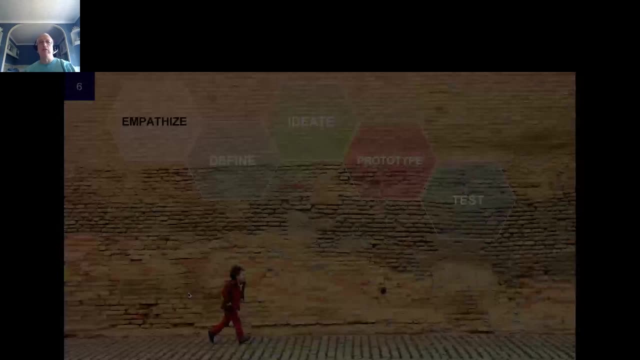 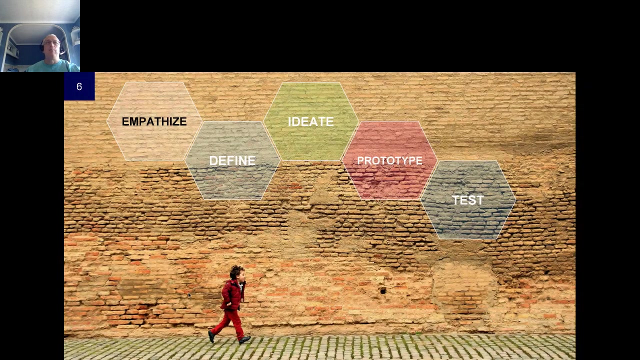 about using a creative technique. design thinking is really important and the idea of design thinking is really important because it's very important for us as a company to be able to do that. the idea that i just presented for an ideo basically has five steps. it's emphasized, define, idiot, prototype and test, and it's sometimes kind of hard to. 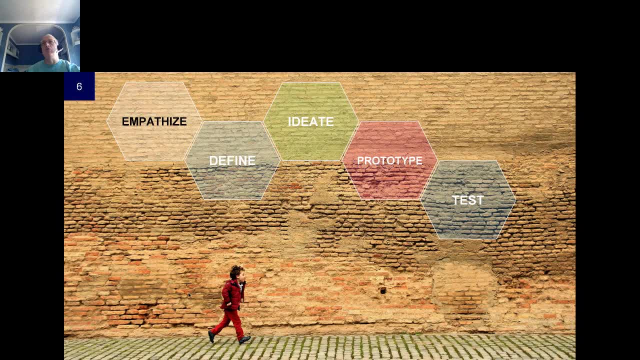 actually wrap your head around what that really means. for me, it's five strategies. that's going to ensure that your product, your project, your change management is going to be successful. it always starts with the emphasize, and we are humans. that means immediately, when we see a scene, we're going. 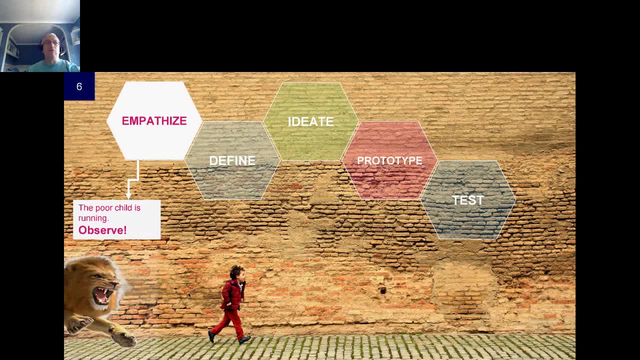 really don't know why the child is running, and bad case would be: there's a lion, so we need to help the child, so we have a problem to solve. and that would be a situation where, yes, we detect we have a problem and continue with a project. the second situation might be the child is just running and 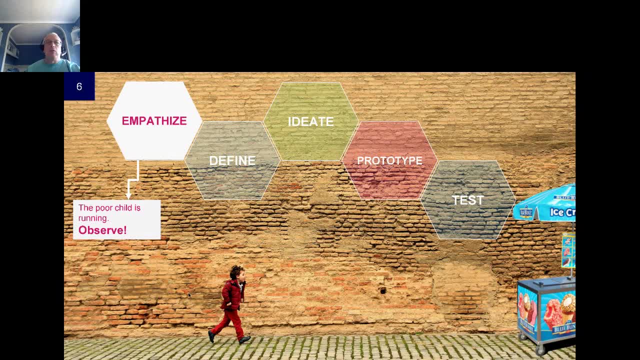 wants to buy an ice cream. well, this is a situation where, well, someone thought we have a problem, we did an investigation, we checked it and actually, um, we don't need to build any solution, we don't need to actually change anything. and the second, uh, let's say the second option or the section. 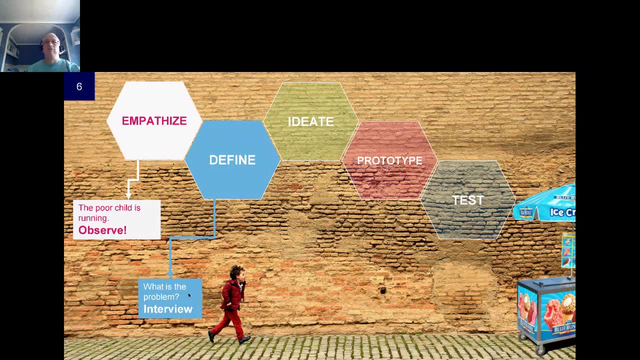 uh say, a benefit of design thing is really this defined phase, so many projects that we see is they're the wrong people writing the requirement. it's the head of, uh the of a department, it's, uh, the ceo of a company that kind of thinks this is the way my employees should work, and while 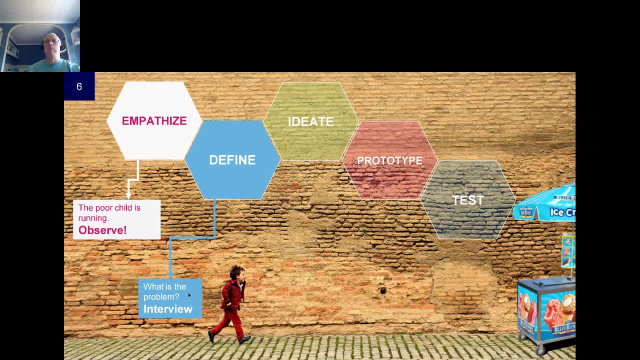 this might all be true from a business perspective. the only way to really figure out how to solve this problem is to find a way to solve this problem and to find a way to solve this problem and to find a way to solve this problem and to find a way to solve this problem. 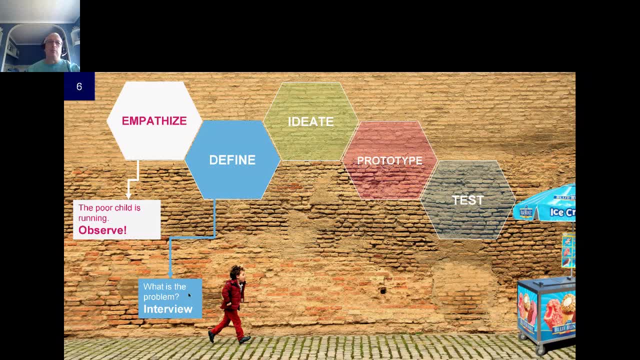 what you need from a requirement in a testing uh perspective. you really have to sit down with those end users and have those conversation. so the second benefit of design thinking is it really forces you go and seek those end users, have those conversations and be 100 sure that what you're 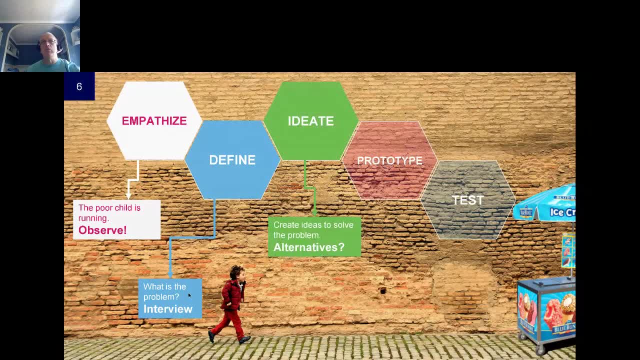 building is really meaningful for them, which brings us to the ideation part, and this again is a stumbling block. often, when people have those requirements to list it out and we have discussions with technicians, they immediately say, okay, this is the way we're going to solve the problem. 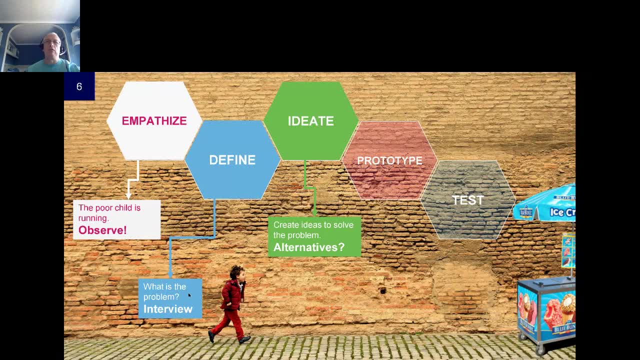 and it often depends on to what company you're going to go. if you're going to come to microsoft, well, we have microsoft products. if you're going to go to sap, well, we have an sap product. and if you're going to go to ibm, well, we have an ibm solution. the point here is: technicians are great. 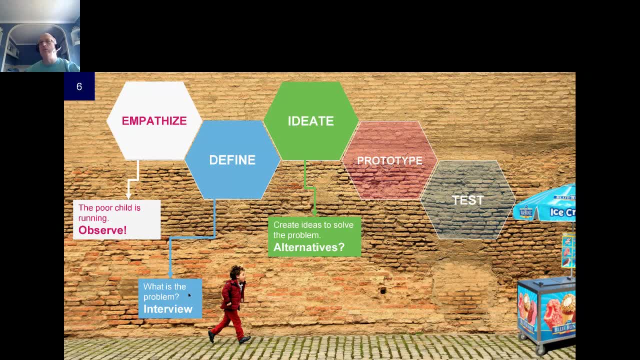 at solving problems, but you should kind of be skeptical or wary about maybe the other alternatives. not only those technical solutions that we have in the ideation part is going to be really important, but also the other alternatives that we have in the ideation part is really about. 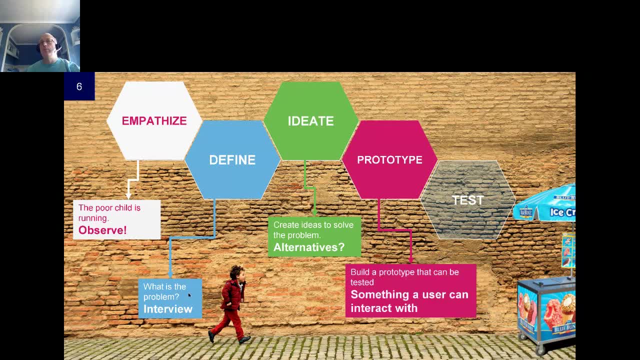 bringing those other people and those other perspectives into the ideation process. and the fourth step is about prototyping and often the misconception about prototyping. what you're going to see in many software development teams- oh, we need a prototype, we immediately start decoding and they build something and while they build a prototype, invest time and then, once it comes to 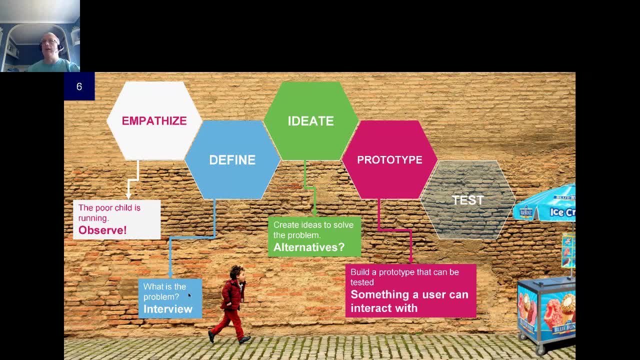 well, now we're building real application. discussion is: can we take those prototypes? do we need to kind the lessons from design? thinking is, a prototype does not need to be any coded seek. it can be a user story. it could be a, a storyboard, a user journey. it could just be walking the end users. 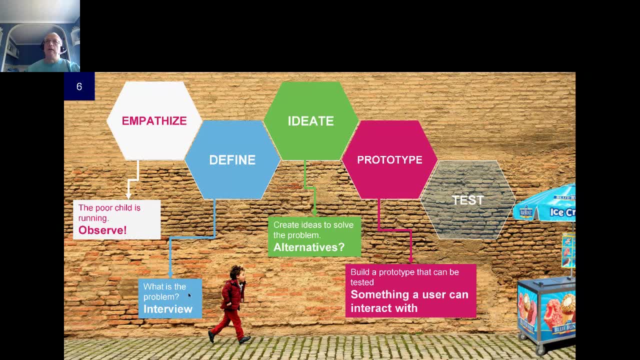 through a situation: is this really what you want to have? and the last thing is when it comes to testing. so in many cases, you might be building this prototype. you're super excited it works, you get a good feedback, but you really don't test it. so you immediately start and jump to the 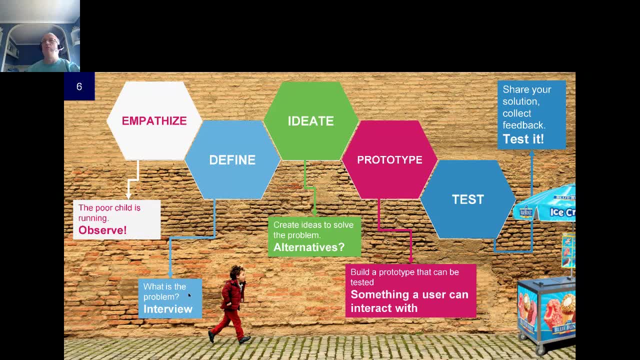 conclusion: the prototype works well, then we can scale it. so the testing is really the last one with ties back to the end users. in the defined state we had to differ- or the discussion with the end user: is this what you want to have? and in the test phase, within testing, does the prototype? 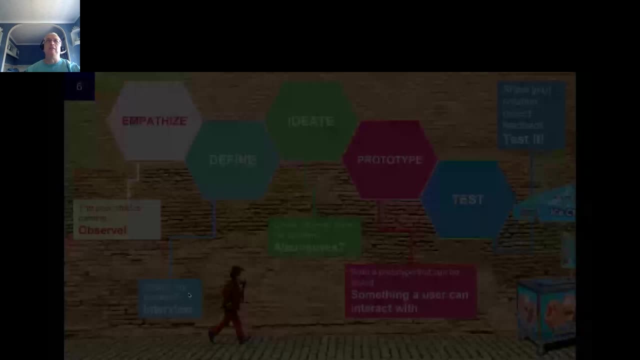 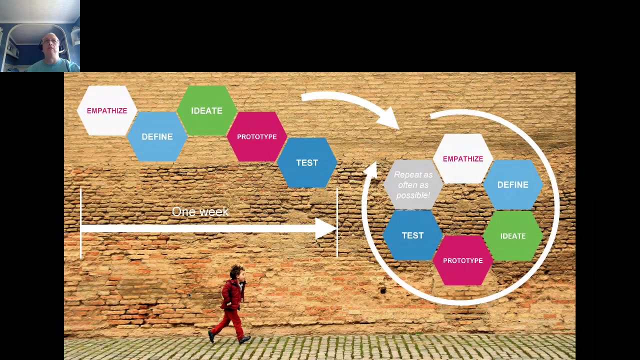 really match expectations. so the nice thing about design thinking is you can do this in one week if you go through those five steps. and maybe one last thing about this is this misconception that in uh use design thinking, you have to start with emphasize. or maybe you're working on a project. 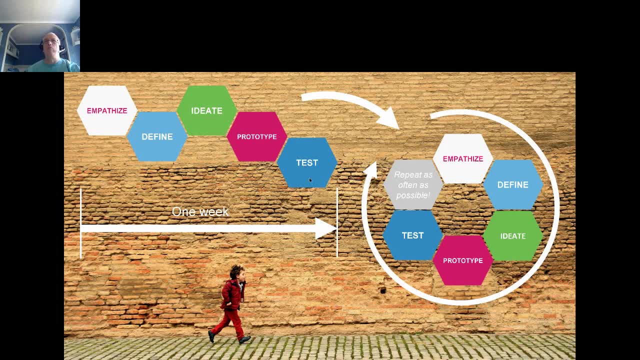 and you're in testing and you're kind of stuck with that and maybe that's the place where you kind of ask your question: are those requirements correct? does that really make sense? and you go back to the emphasize the phase, and then you question the define phase and then you question: 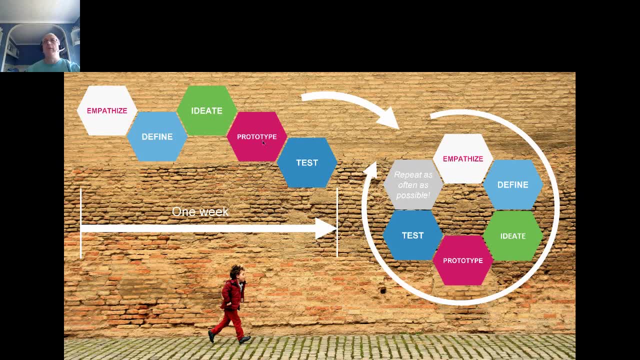 the ideation, the solutions and and the prototyping. so the message is: think of those five um uh activities as as opportunities for you to ensure that your product uh, that you kind of deliver, and then the end of the day is really going to be successful. you don't have to start as emphasize. 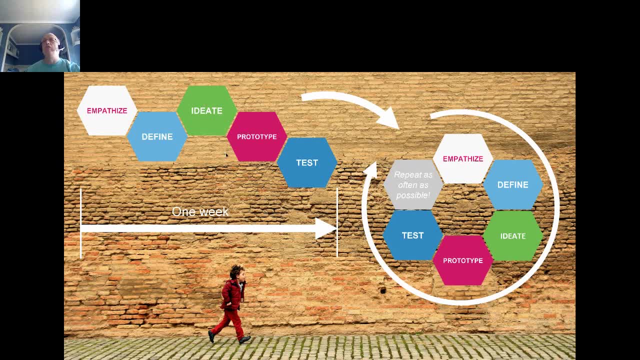 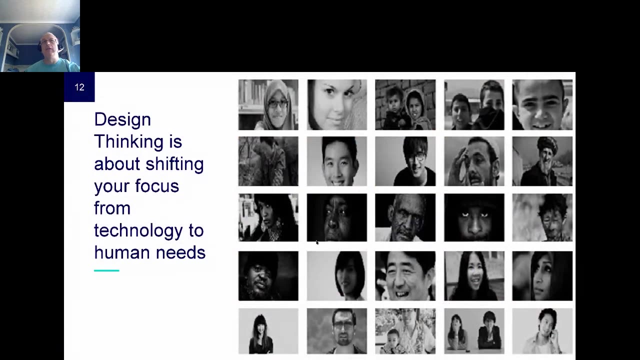 you can basically start at any phase, but just ensure that you really have a clear understanding of them, and in most cases it's an iteration, so you might start with a smaller part and and evolve your applications over time. next step, about design thinking. we live in a technical 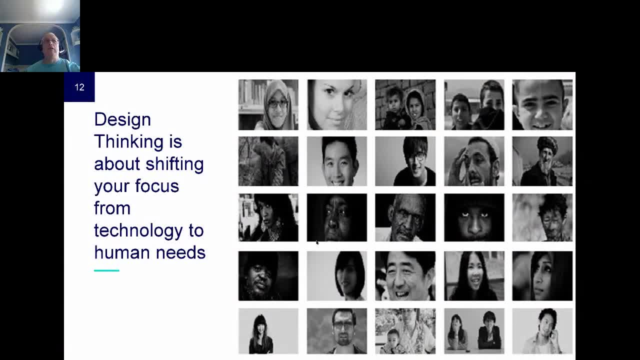 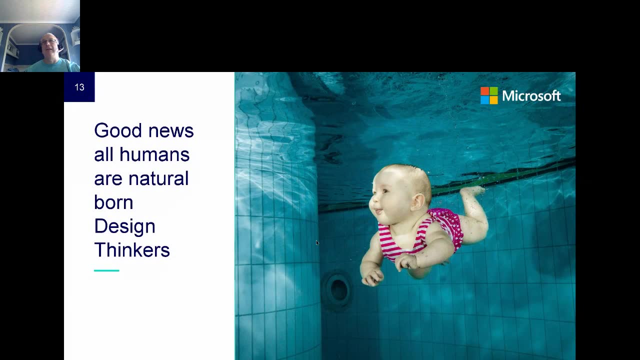 uh, society and we all love technology and in many cases when we have problems, the first question is: like how can we actually apply technology? but the learning from design thinking is: maybe you want to go one step back. and that brings me to the next thing is: can everyone use design thinking? 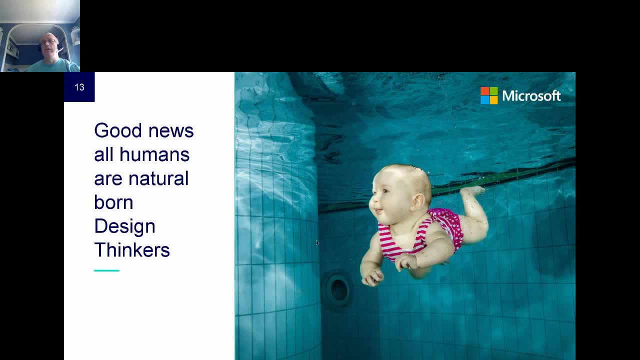 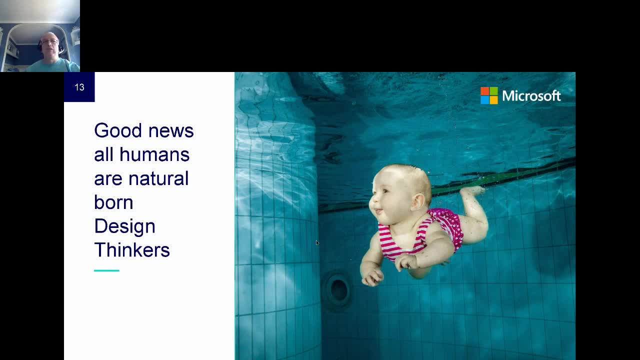 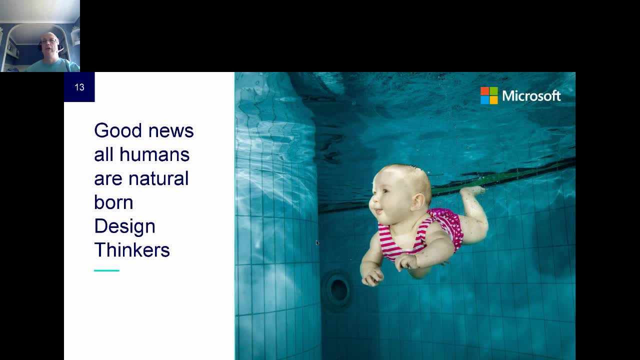 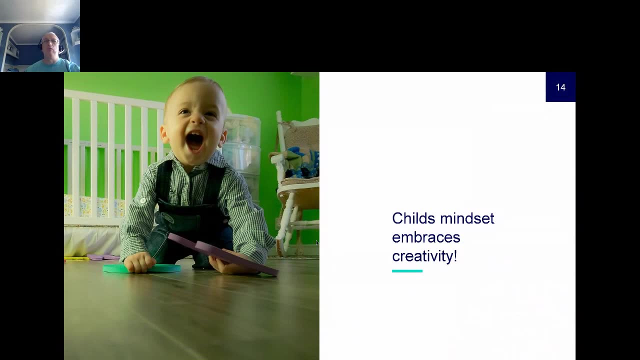 design thinking. i'm not sure how to do, i'm not sure how i can actually implement this head to head play, so I'm passionate about it. you know, for me, when i was watching a movie- and i don't know why, but i wasn't even looking at the air保 most of the time- energia was acting very añadiemente edition, i sort 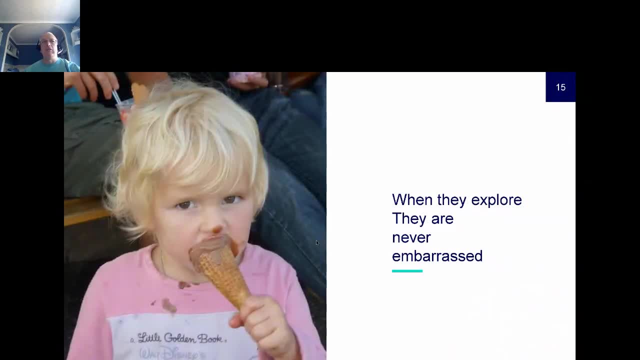 creativity. but then also the other thing that's nice about children is like they're not embarrassed to try out everything. if you're looking at this child eating the ice cream from an exploratory point of view, that makes a lot of sense. or you can feel the texture, you can feel that it is cold. 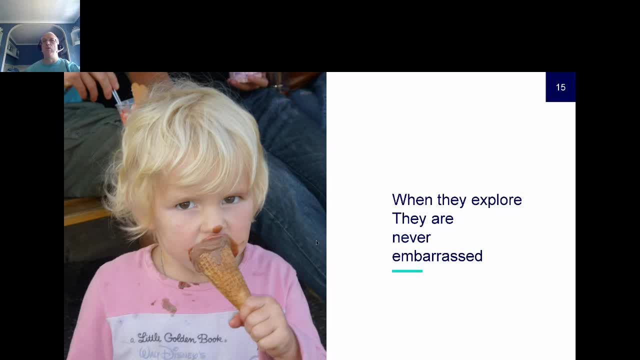 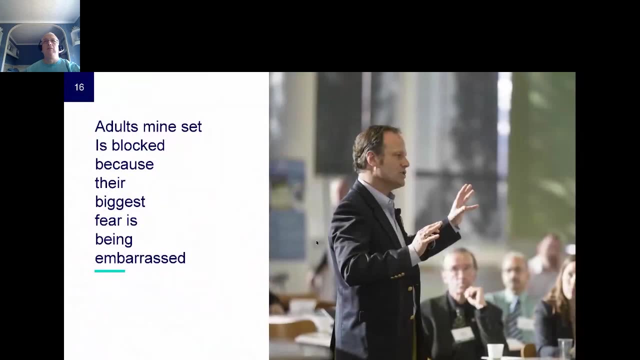 it's smelling the ice cream, tasting it all at the same time- would have grown up to this. uh, when they're exploring, no, they want in general, and this is actually awesome barrier. and this brings us basically to the cultural limitations that we have in organizations and why designing is really 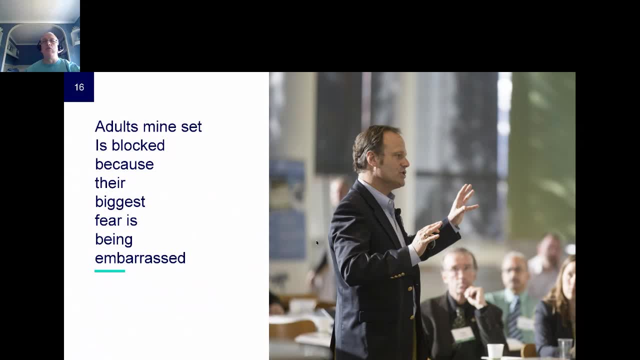 helpful for all kinds of changes, from change management to innovating new products or kind of finding new ways of working together. it's really that people are embarrassed or they're feared within- uh, within an organization hierarchy. imagine that you're called into room with the ceo and someone's asking you: well, what's your idea for solving problem x, y, set well before. 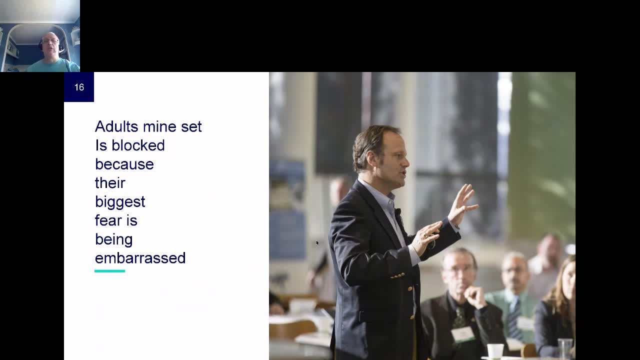 you raise your hand, you're going to have all kinds of faults is. is it appropriate to say it? what if people think my idea is stupid? what is my line manager going to think, oliver, bring these ideas up here. people might just think that i want to shine in front of the ceo. i might be offending. 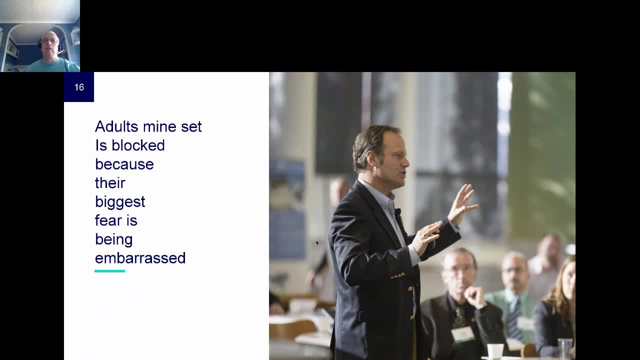 other people with my ideas against something that's uh done in the organization. so there are hundreds of reasons for people to actually keep back with their ideas and improvements, and that means you don't have those ideas when you're trying to improve processes or projects, uh, or or working on new ideas. and if you look at those two pictures, 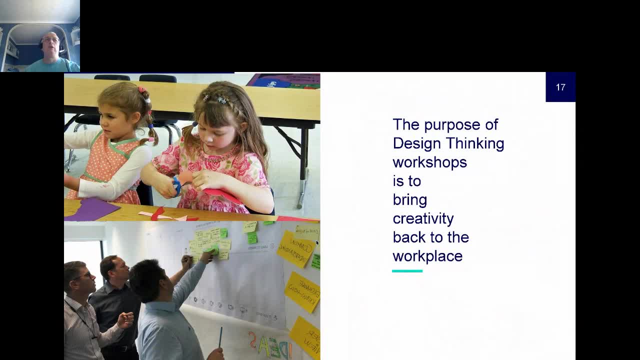 you see those, um uh, two children on the top and the three guys on the bottom, and on the top you see them in the kindergarten and on bottom it's a design thinking workshop. the message here, essentially this, is really exactly the same thing: a kindergarten is a protected space for children. 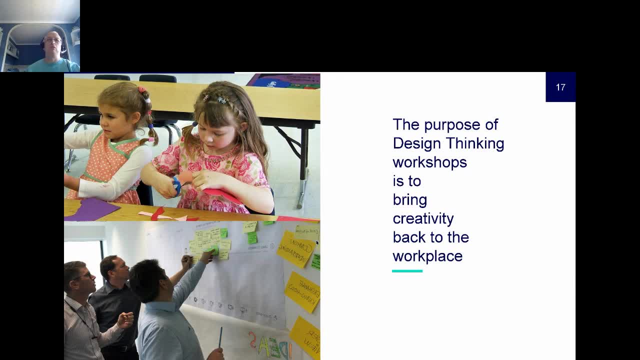 to be creative and no one's going to ridicule them and point fingers at them and laugh at them. if a child draws a cat with five legs, no parent will say you stupid, because a cat only has four legs. they're gonna have a conversation and open with their kids or they're gonna find it very nice. 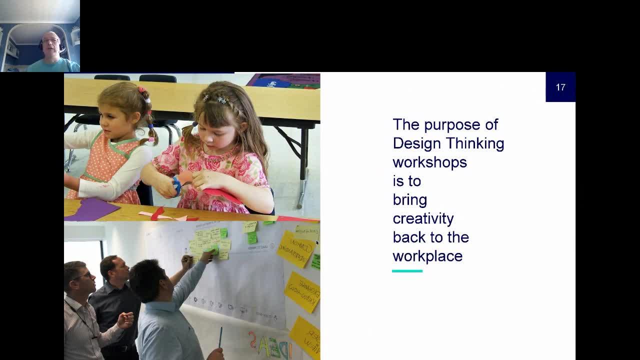 so, and the same thing is about the design thinking workshop, the idea of a design thinking workshop. you have this protected room, you have this protected event time box, basically for three, six hours or maybe for two days, where everybody can share all his ideas without having thoughts that mean: are people gonna laugh and it's a team exercise, design thinking workshop? no one actually. 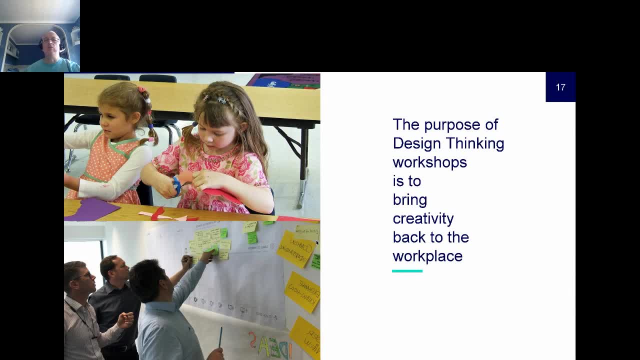 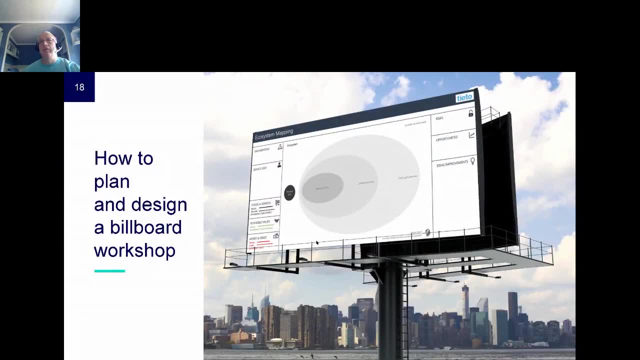 cares who has the ideas. they're successful if the group together can actually solve the problem. they said um as an introduction why we need design thinking in organizations in the beginning, kind of linking to those two scenarios where you can use design thinking in requirement engineering and the other one is change management, crafting your 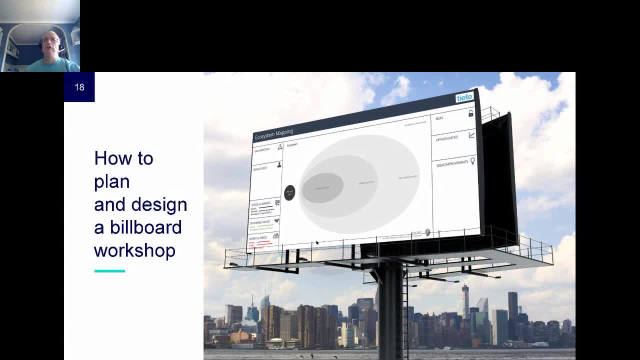 project strategy. so, again, if you're a building manager, you need to put yourself in charge of the testing process, improving your test capabilities to strategy. well, our work issue is how you can use this method actually to create your own workshop, and also some tips if you're running this workshop. 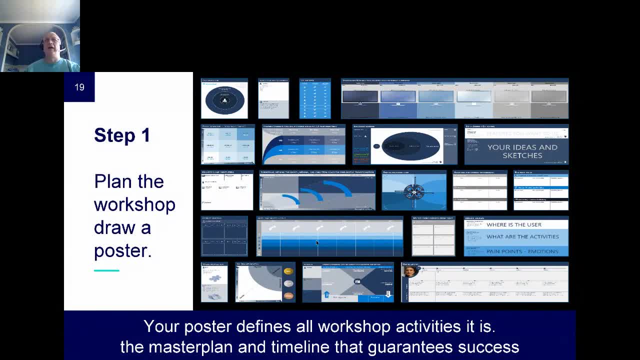 how you can make it successful. so then i think, their free templates. i share them on linkedin. you can download them. in a sense, each of those templates is a task like, for example, stakeholder mapping is like who's involved in my project who didn't need to consider if i want to build my 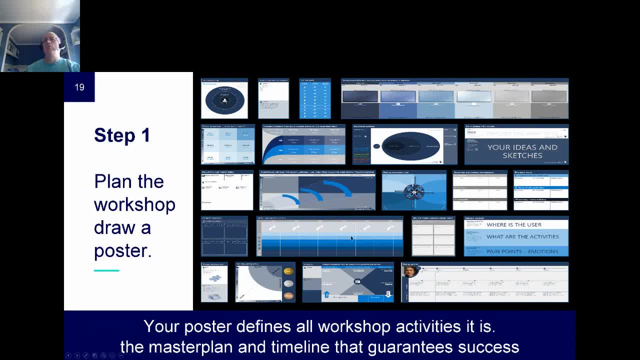 my testing strategy. you might have a user journey, for example. how are you building this strategy? how does this product look like? and there are multiple templates. i don't want to go into details. you can explore them after- but the idea is that each of those tasks are time box tasks. 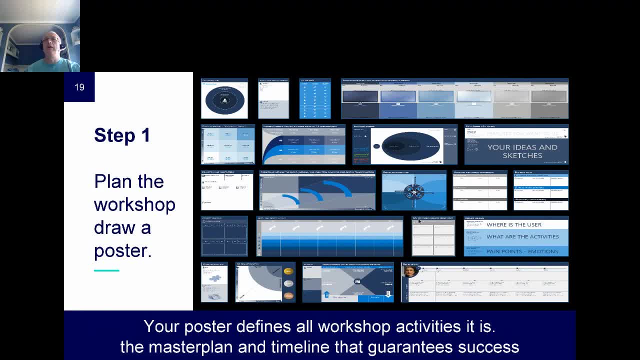 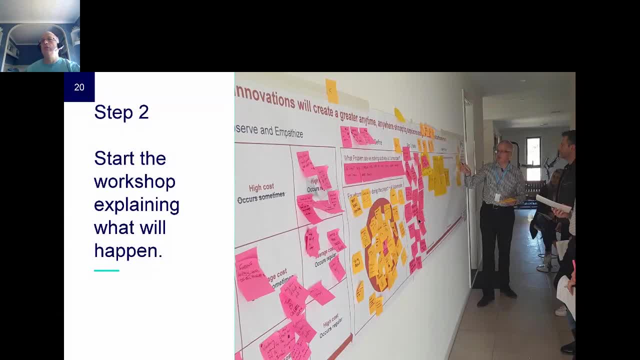 that have a very clear message, a very clear outcome and create something that you can use in your workshop. so how do you start your workshop? you create your poster. you do this in powerpoint, you print it out, you hang it on the wall. this is an example of a workshop we did in australia. 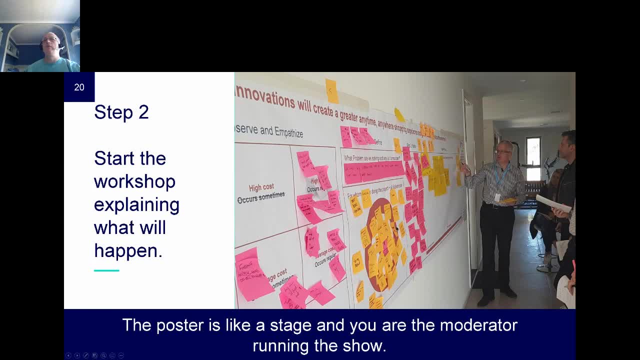 and you just walk the people. well, here we're starting with some emphasizing, then we have over here we have some stakeholder mapping, and then we're looking at a process and, on the end of the day, before we leave the workshop, we want to have a clear understanding of the next step. so 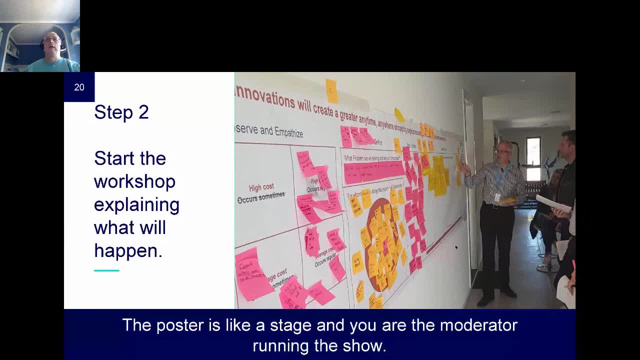 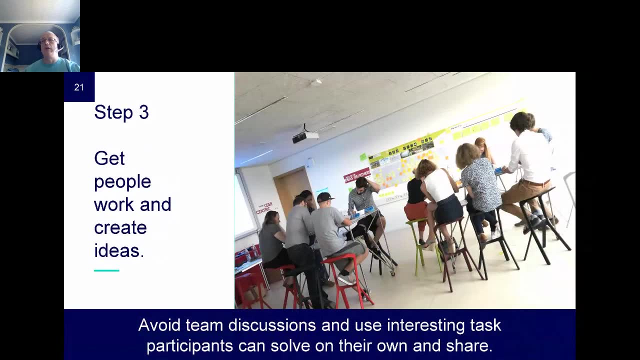 this is typically the way you're going to introduce a workshop. then the question is: how are you going to start your workshop? and many people, uh think workshops is much about discussions. i try to remove those discussions and my first exercise is always going to be a task we call it alone, together meaning. 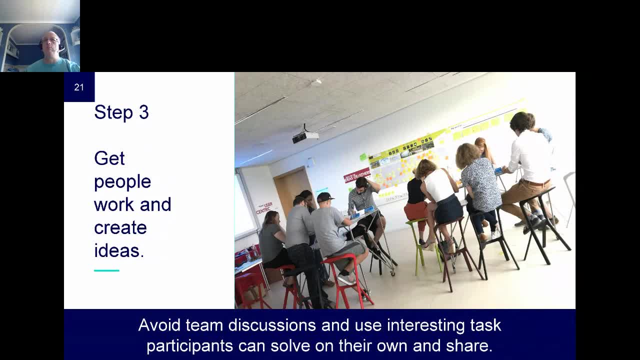 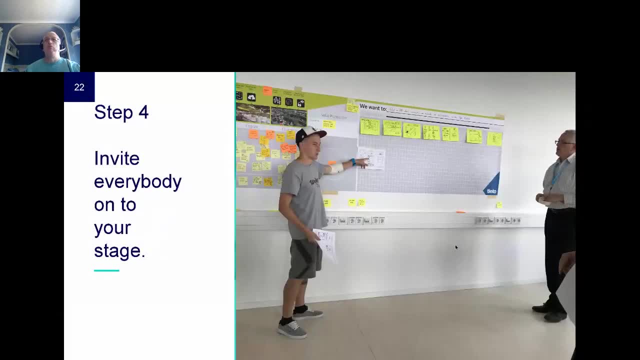 people are going to get five or ten minutes to think about a problem, to think about solutions idea, and then they're going to share those ideas one by one and, as i said before, it's really about enabling everyone in the organization to share your idea and, as a moderator, what you're trying. 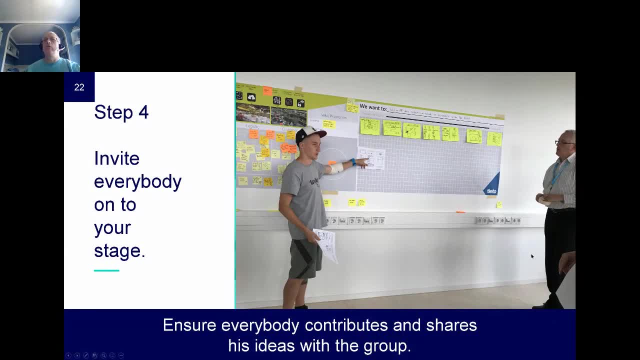 to do is: here's your poster on the wall. you're here as a moderator and you're trying to kind of give those people a stage to share your ideas, and often people- you will find different kinds of types. some people are really keen to share their ideas immediately, are going to jump up and 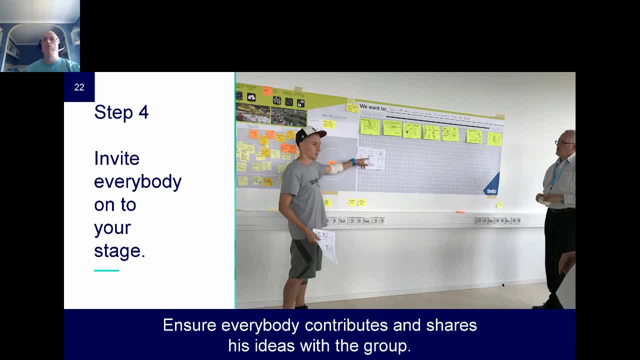 say: this is my fantastic idea. other people are going to be more shy. so your role as a moderator to get out those results in the workshop is really to bring them on stage. make it clear that everyone should be listening to them. um, help them so they feel secure when sharing their idea and ensure 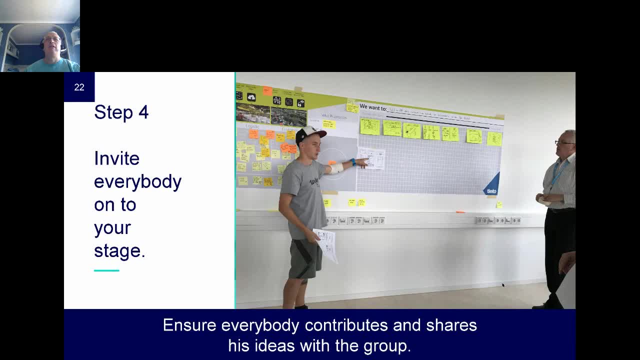 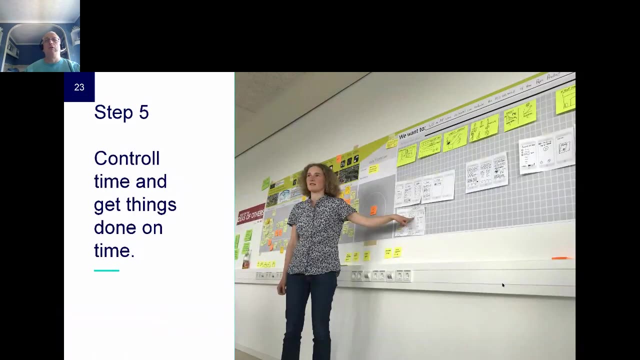 that everyone in your workshop is sharing your ideas, not only those people they're self-promoting, that like to stand in front and uh and talk a lot. really seek those quiet people, because they often have contributions that are really outstanding. the second thing, or uh, when, when. 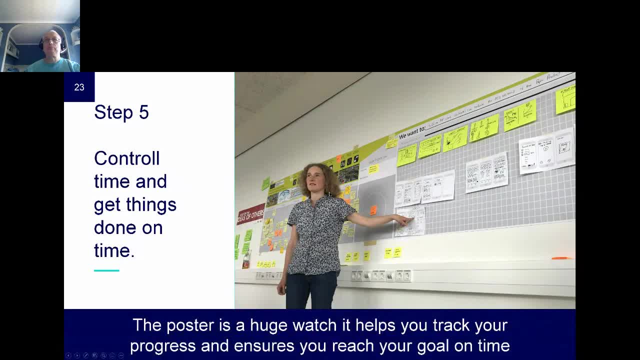 you kind of use this approach for design thinking is. i see this poster and this is virtually as true as in a physical workshop. it's like a big progress bar. so you put up kind of on the top some stickers how much time you're allotting to these individual activities. 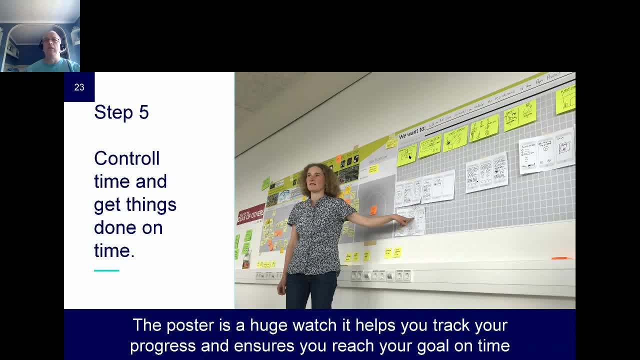 because you really want to ensure you can complete the workshop on the end of the day or in the time that was given by the team. sometimes you have a top level managers or you have people that need to bring the chair or pick the children up from kindergarten, whatever. so if 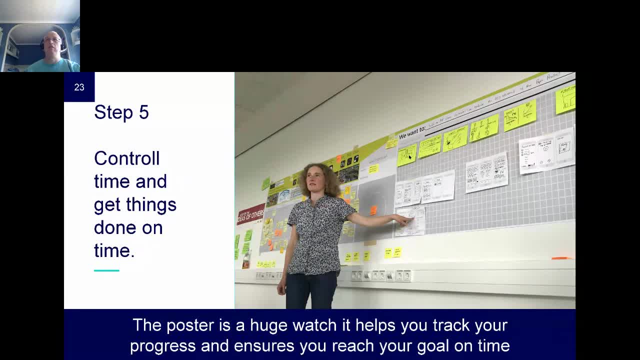 you promise to deliver the workshop by four o'clock. you should be finished and they're having an overview and a good plan and the timeline is just going to help you to ensure so you know are you in time or not. then in workshops in general, you always have to also. 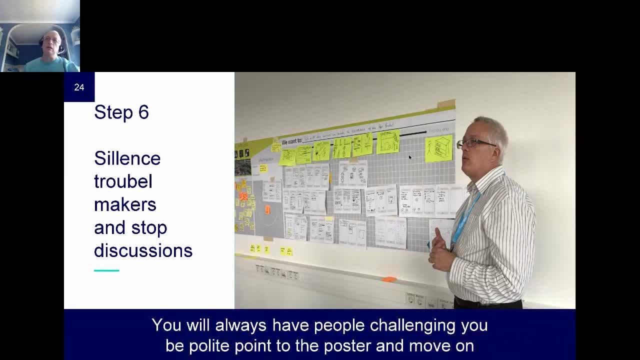 think about how you're gonna um deal with troublemakers, and what i mean with them is like people that are maybe kind of higher up in the organization. they're just used to talking long and and having more year on the time, and what you're basically doing is, since you're controlling the 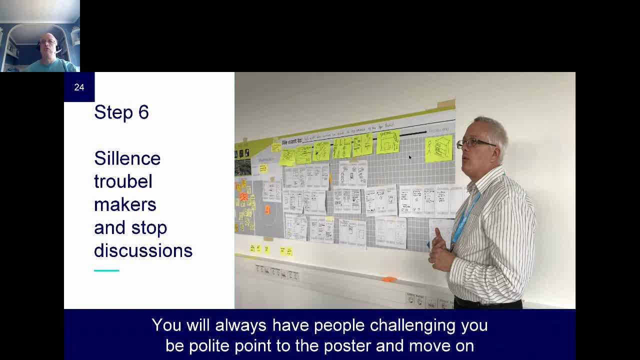 space and this is your poster and you're running the show. you're just going to tell this person thanks for your contribution. you're just going to tell this person thanks for your contribution. you're just going to tell this person thanks for your contribution. you can ask someone else to come. 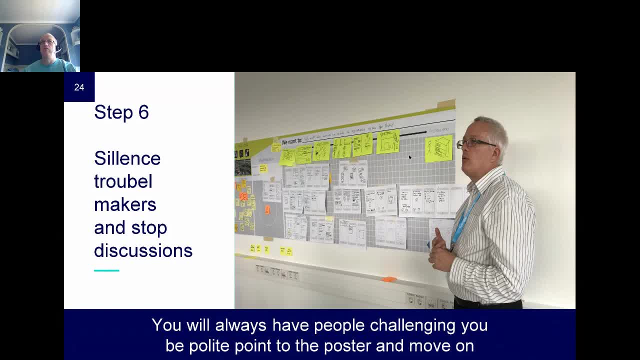 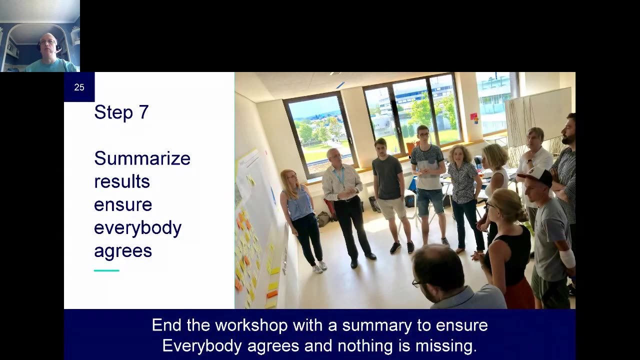 and share their faults. you can do this in a virtual online as well as in a physical online workshop, but it's really ensuring tool that everyone has the same ability or the same time to actually talk in your workshop, a nice way to close all of those workshops and that's also important. um, it's a big ass from an. 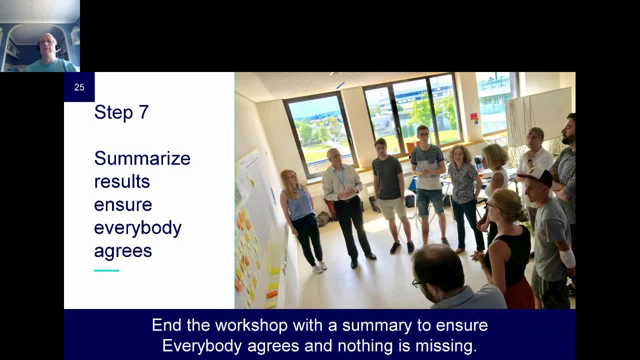 organization, you might have a larger team. so i want to spend a full day or one and a half or two days with a team. and i want to spend a full day or one and a half or two days with a team- and that's with a team. and i want to spend a full day or one and a half or two days with my team to craft. 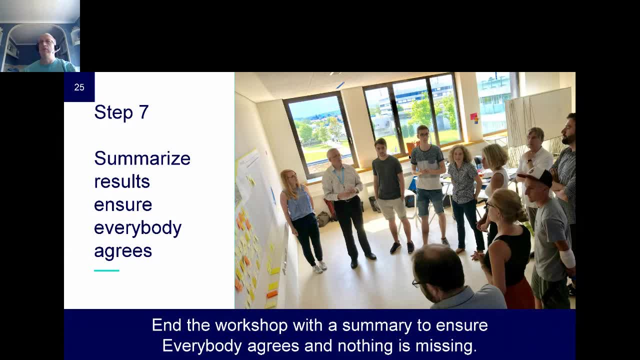 a new testing solution. so what are you giving back to the organization? i mean, if you have 10 people and you have two days, that's basically 20 men days. this is like two-thirds of a month, yeah, so why should management do it so? very important is a summary. 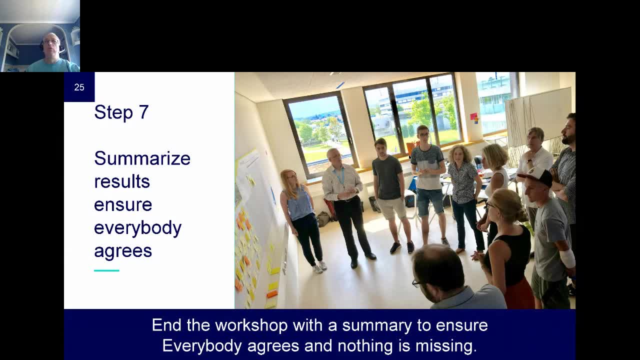 from a workshop. it's always good to pick out a person who's going to walk you through the complete uh summary. what you did, like we started with looking at your personas, then we started to look at what are actually your real problems and then we started to look at what are actually your real problems. 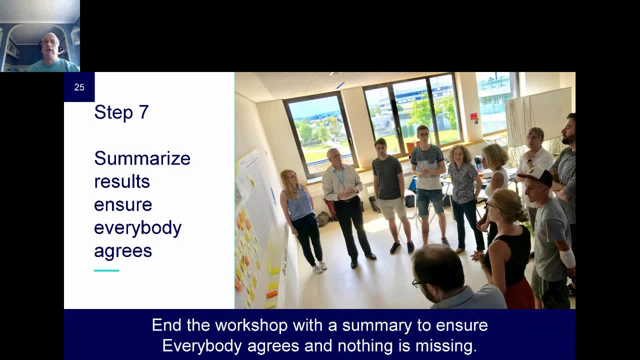 uh, in the test environment, uh, maybe we detected some misalignments with the development or the product owner. kind of give a complete summary of the story for everyone who's in the workshop. why? because the next day when they go back to the workplace, the first thing people are going to 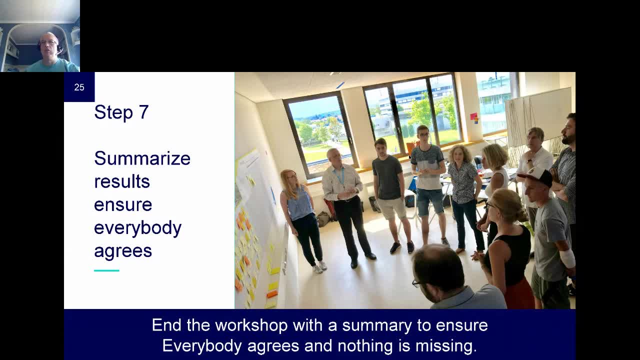 ask: well, why didn't, why weren't you here at work yesterday? oh, we had a workshop. well, what you do? the last thing you want them to say: oh, we work up kind of writing post-its that kind of sounds like it's not work. so what you're doing is: 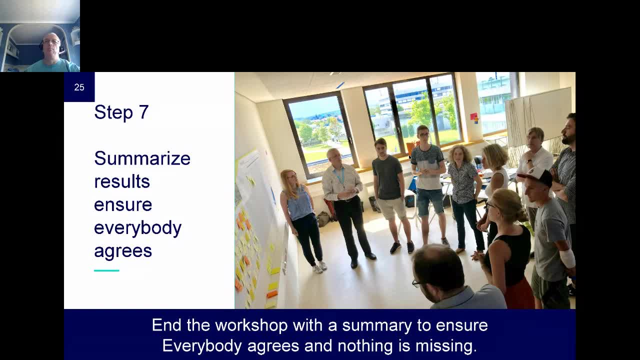 you're framing a story that they can bring back to the managers, to their colleagues, and it's also kind of a final verification. we all agree that this is kind of um what we discussed in the workshop. the last thing, that's also super important and i'm convinced the workshop without 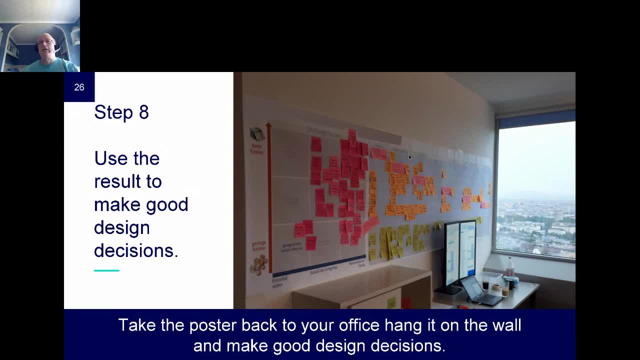 documentation is really a waste of time is after workshop is finished. uh, the workshop owner should actually uh sit down and write the proper documentation. why? because in many cases you will have good, innovative ideas. you'll go to management say, okay, we had all of this discussion. the best thing would be we will go in by the following testing tools: we will create new testing. 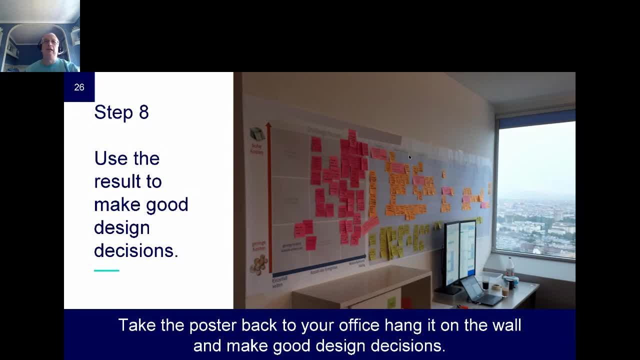 teams. we need to hire another three or five people and they might say, yeah, that's all fantastic idea, but uh, it's september, so let's have a conversation next january, or no, forget about january. we have a new project to come back in march, so capture all of those information. it's a valuable you need to. 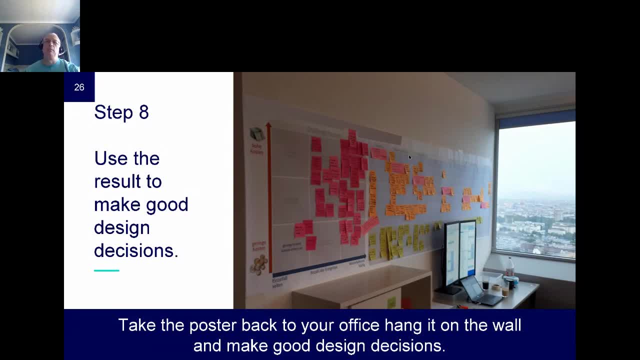 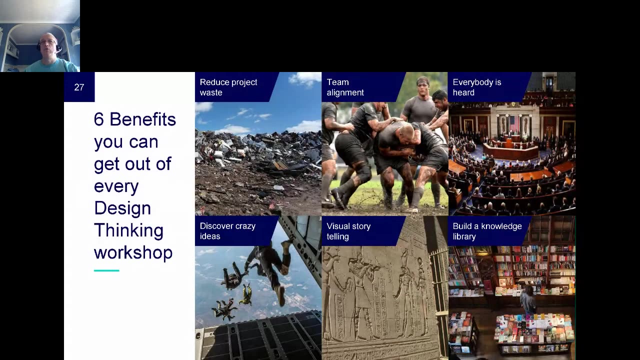 and need it, basically, uh, whenever you get okay from management, from from the investors, from your client, to actually jump start the project. the last thing i'll, um, just uh talk about and then i'll go into a q, a, six things that you can get out of your design thinking workshop in general. 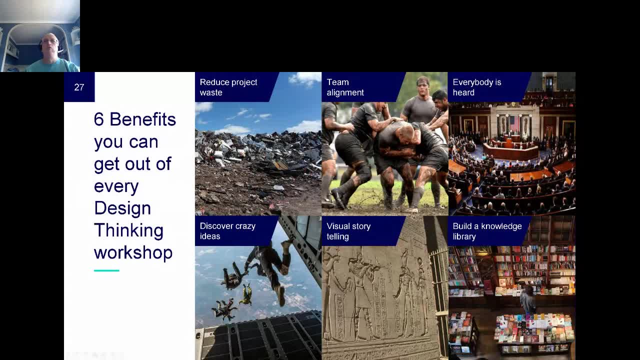 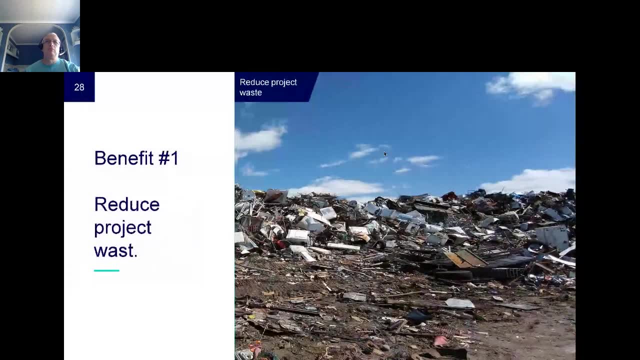 and the first one might not be super obvious, but the first one is really about protecting the environment. why? because, um many cases you have many consultants flying over the world, traveling, spending huge amount of energy, and we still have like 40 of all software developed, isn't there, never goes into production, so huge amount of effort and energy wasted. 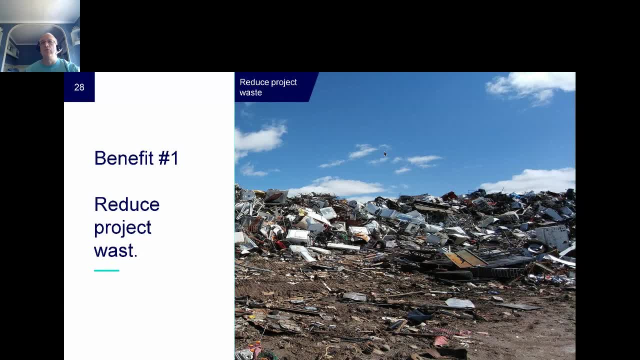 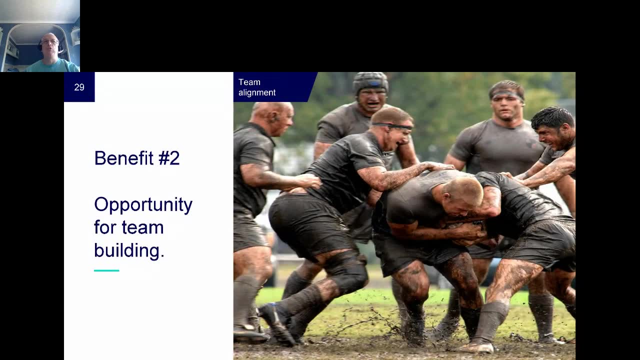 and design thinking can kind of protect you from working on projects or creating projects most probably won't be unsuccessful. the second important thing is really about team building. this is for your internal team, but also for customer projects and many projects. the first time, let's say you're going to have to account. uh, 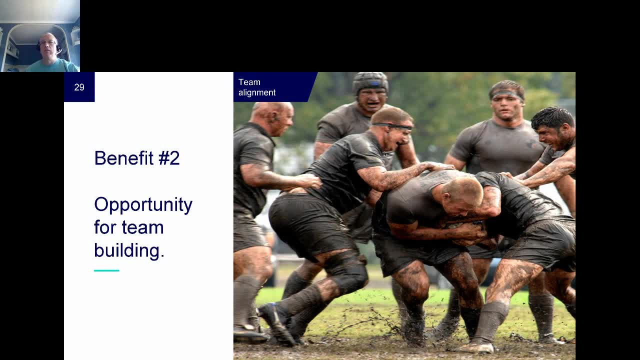 or the customer manager working with the factory manager and sitting with the warehouse manager employees in the same room. take this as an opportunity for team building. when you're trying to craft a strategy, trying to craft a project or trying to craft a change management initiative, take this as opportunity to have those people sit together and exchange ideas and better. 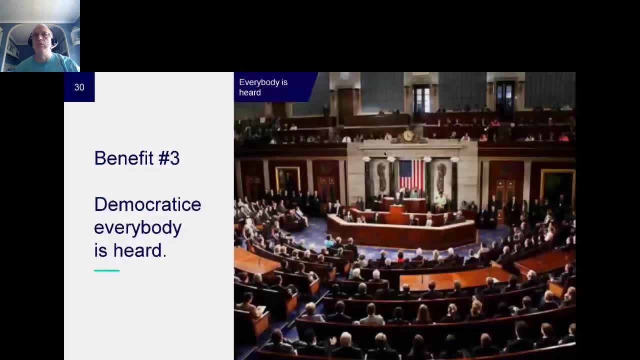 understand the views and why things maybe are not working in other departments when it comes to team building or what some of the skills are to take a challenge and solve a problem. so this is what i'm going to be talking about. um, what is an impact of a team building you? 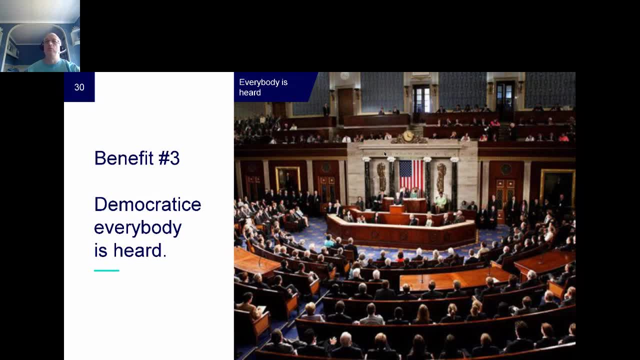 have to think about this in order to really be successful and engage your audience, and you have to think about this as a Agile community, and both the teams should be in an Agile community and it should be fully engaged. and then the team isn't, and so you. 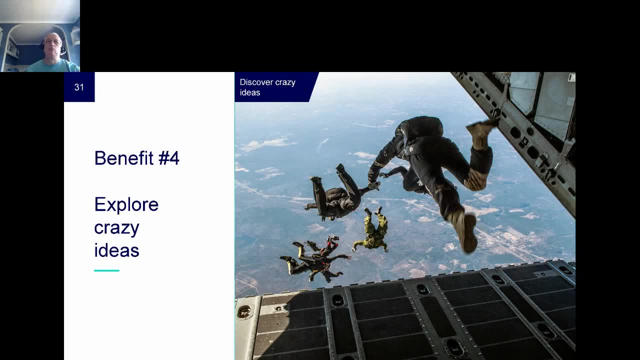 need to be really involved in this and it's necessary for the organization to be active. Let's be super crazy. Let's go in and use Bitcoins for, let's say, a purchasing process, And people say I'm not sure if that's a good idea. 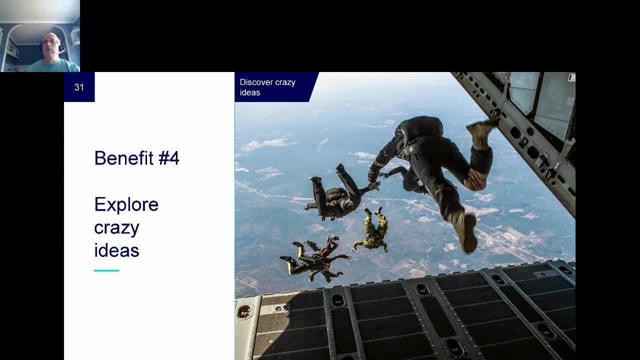 And someone raises his hand and says: you know, my friend, my colleague is just creating or writing a PhD, And that is an expert. I just can call him and he'll be here next day. So it's really about people sharing all the experiences from the life and saying, well, those are things we could actually do. 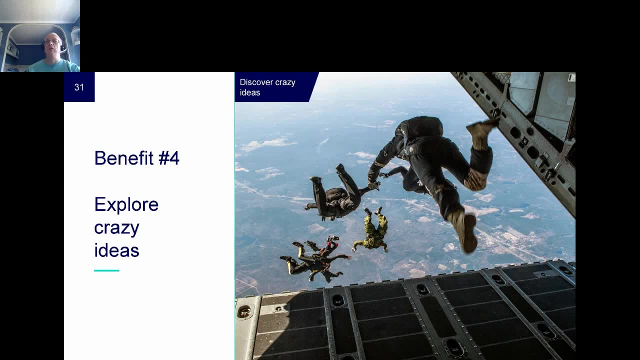 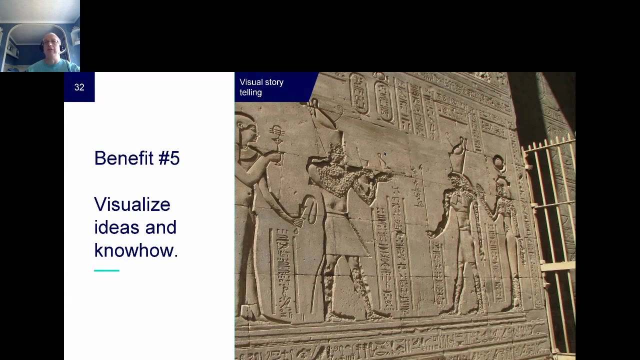 And if you know that someone in the group has this ability, this knowledge to share in the project, then often that's kind of a starting point for people to really think about this as an opportunity. The fifth one is about visualizations. If I speak something, if I say a word, it's like it vanishes. 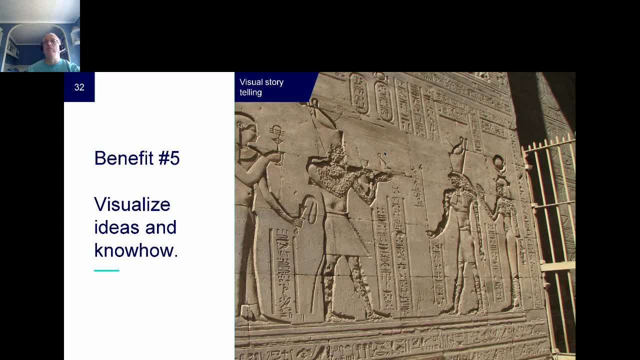 It's gone The moment you write it on a post-it, you can move it, And this is just an example. If the Egyptians didn't take the time to chisel all of that in stone, they probably would not know too much about it. 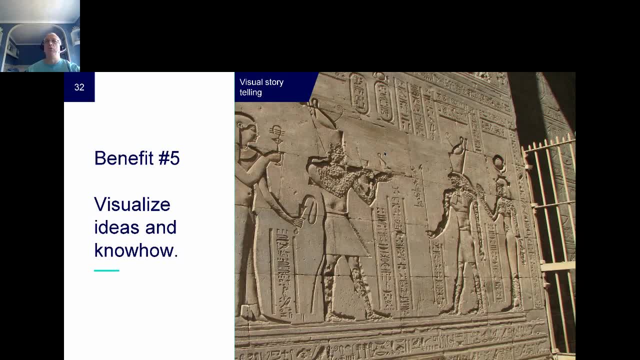 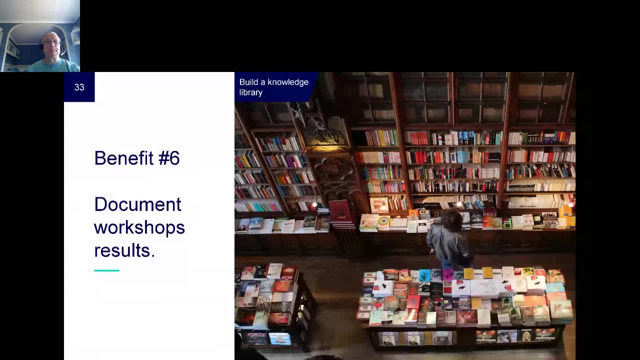 And the same is true for a workshop. If you don't document stuff, if you don't write it down, it's the information is basically lost. And the last thing is really about benefits of documentation. If you're running those workshops, it's really a unique insight and opportunity. 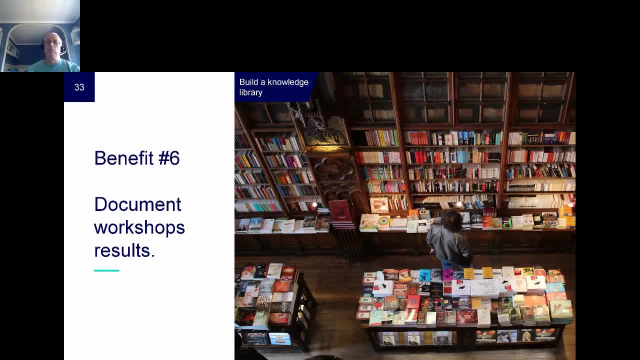 as a consultant within a company or with customers, to really listen and understand those details about processes, about the process, the products people want to build, And if you document it, you're really building a library of knowledge. So if you attended or if you have moderated several hundred workshops, 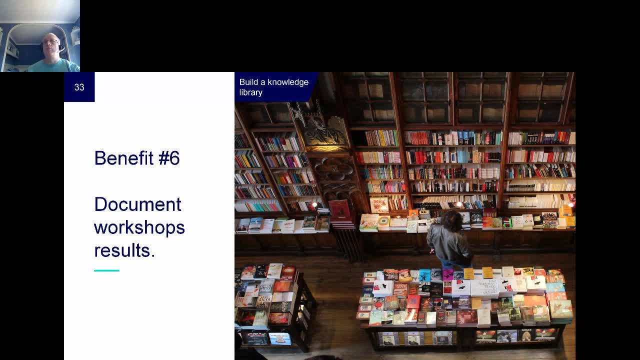 in different industries. guess what? You're building a huge knowledge repository and you start to see, let's say, interlinks between different industries, between different products that you're building, And that just makes you so much richer as a consultant And with that knowledge you can help them in return. 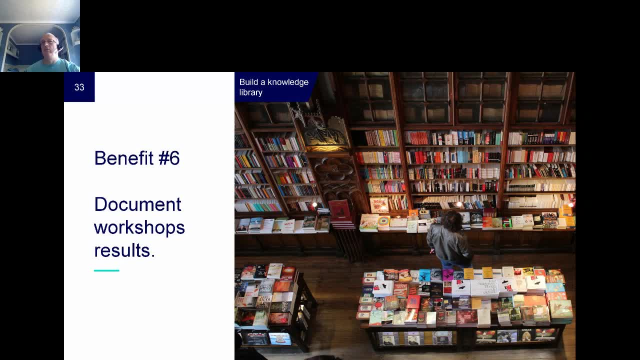 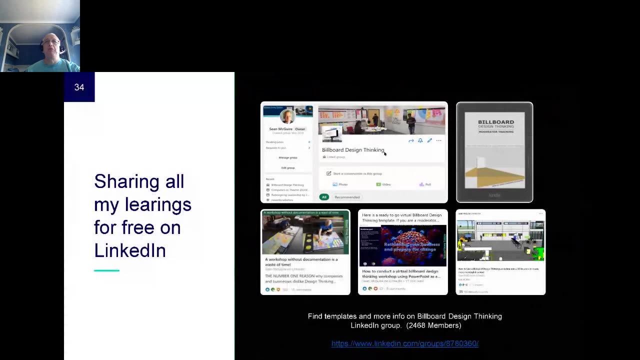 If you have new projects or new projects you're working on, or processes or change management initiatives where you're helping, you can take all of that knowledge and help those people in the groups to guide and build applications and solutions that are successful. This said, I share all of my stuff on LinkedIn. 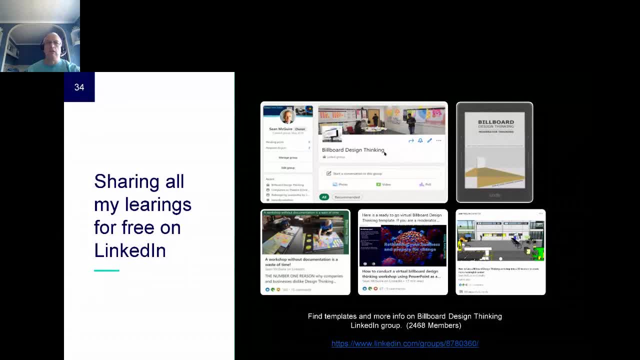 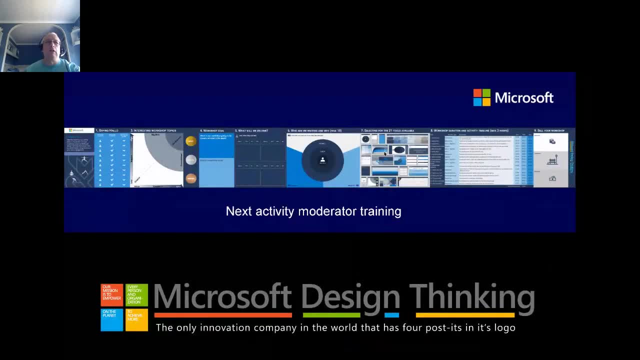 Most of the templates you can download. I like writing articles and like engaging with people. getting feedback on that. Yeah, maybe just the last thing kind of to think about when I joined Microsoft. for me it was like a design thinker. it's really the only company that has four post-its in its logo. 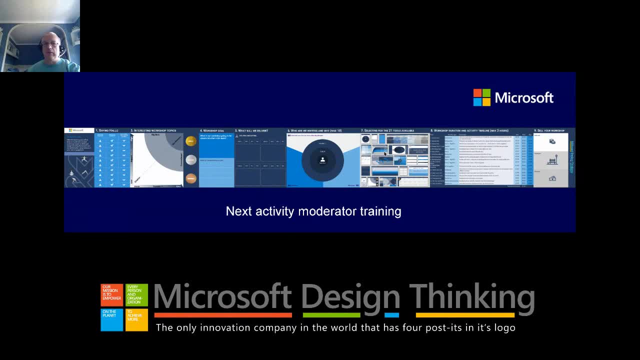 And with that I'm finished with my presentation and I would be open for any questions. Thank you very much, Sean. Let's see the questions. The first question from Andreas. As you said, a workshop might be a hard sell, depending on the company. 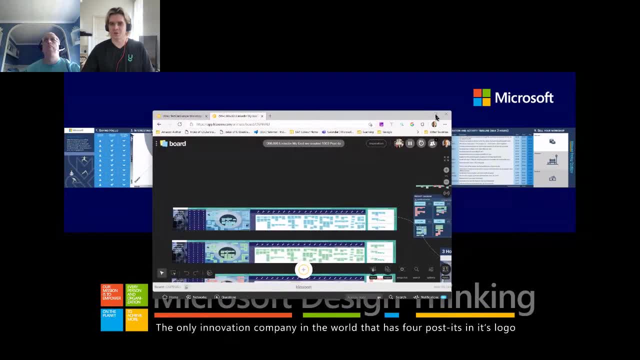 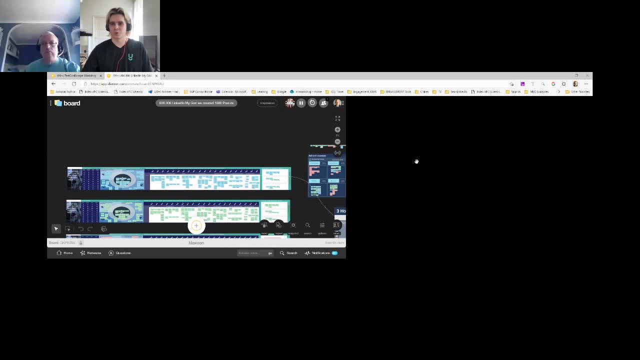 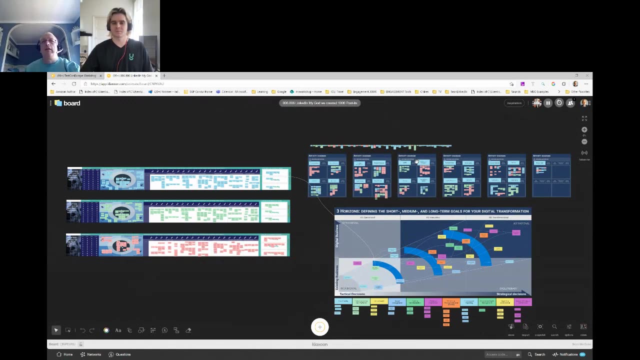 How would you include some of the ideas presented here into daily work, where teams often have more autonomy? What should we focus on? Yeah, so when it comes to building a workshop into an organization, the biggest stumbling block is, let's say, if you're really pressed and you have. 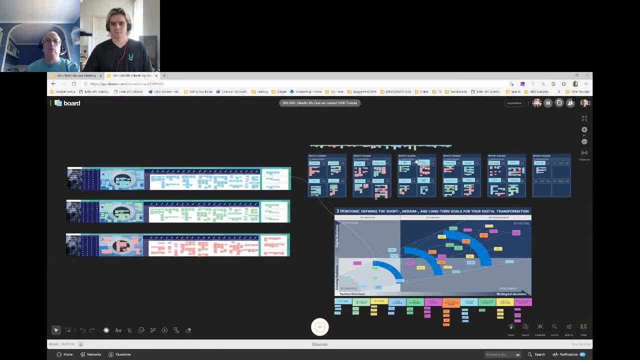 little resources. going to management and asking them for a full day workshop could be like a real challenge, But a workaround is in many cases is those workshops can be also super short. You can have a 60 minute workshop and you don't need 10 people. 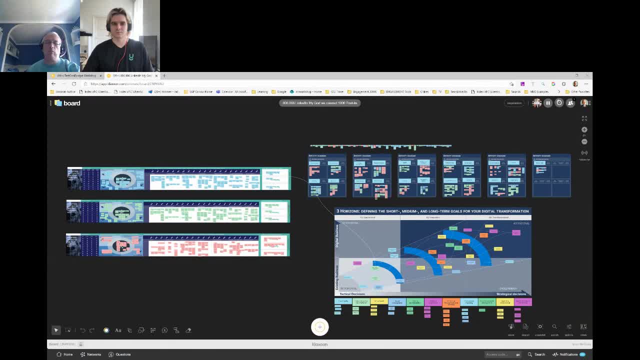 So maybe you're taking five testers or two testers, two developers and a project managers and you just spend one hour, one and a half hours And then you actually show those results to management And what they kind of understand is if they compare. well, 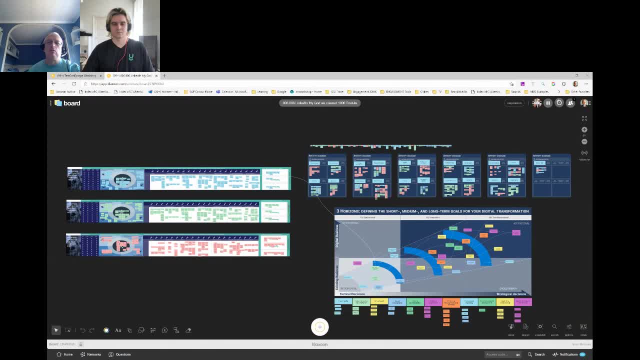 if you have a problem and you're sitting down in one hour face to face or online meeting, what are the results? but now you're comparing it with the creative results from the workshop, so that can be a way to actually sell it into the organization. 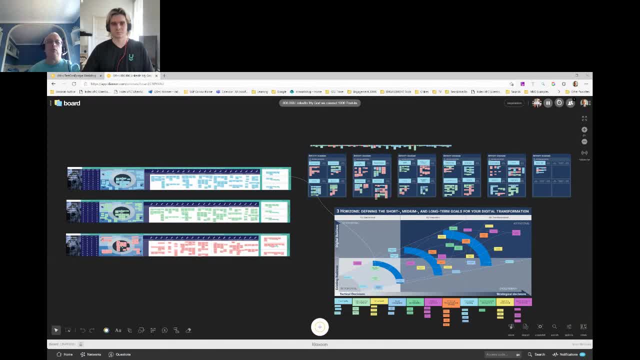 In the end, management will always support you. if they understand that the time that you're using in the workshop is more valuable, Then having a standard conversation, which you probably have every day in daily meetings. Thank you very much. Looks like there is no more questions yet, so we can. 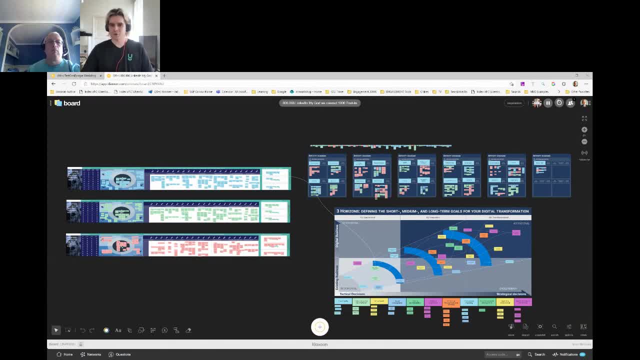 Oh, there is now one. The question is how much time it would take to prepare and organize such a workshop. Yeah, in general, to prepare a workshop, you can say it would take probably one day. I would say eight hours. 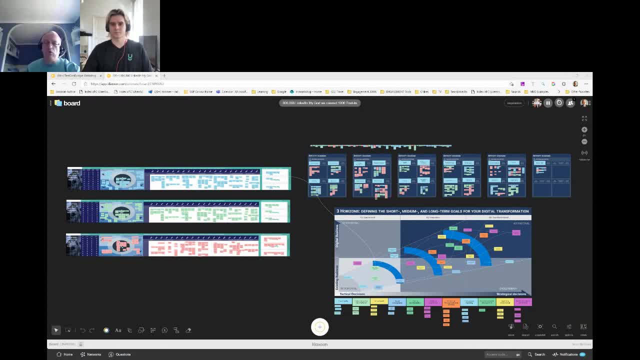 And again, it depends if there's a customer workshop as an internal workshop. So the tasks that you need to do is you need to identify the workshop owner in the organization or the customer. You need to sit down with this person, explain to them what you're going to get. 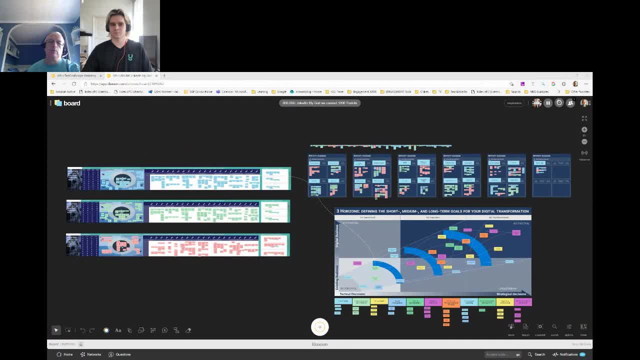 In general, the way I do it, I'll always design a poster, put it into Klaxon, have a conversation with the workshop owner, run them through the complete workshop, start to end. So this is the topic, what we want to do. 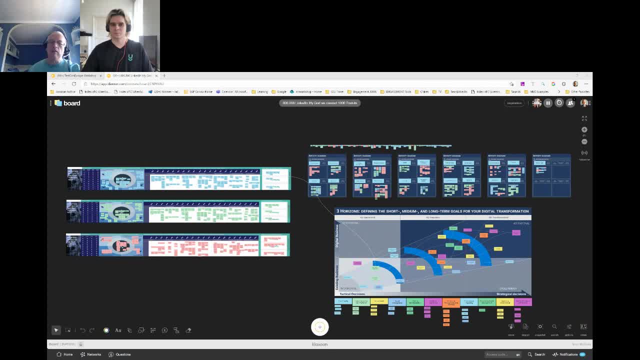 These are the activities, what we want to do. This is the result you're going to get from the workshop And these are the people that I want to have in my workshop. So this is something that usually takes, let's say, one day to set it up, because you're going to have two or three. 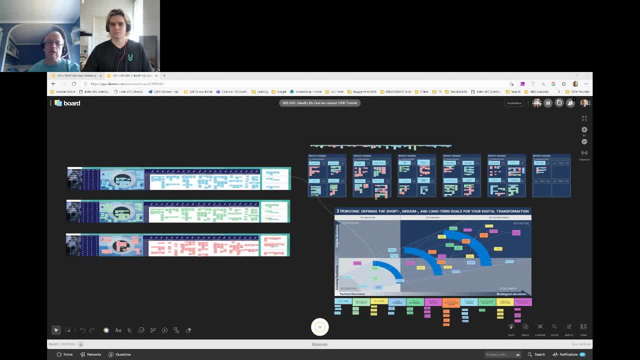 meetings: first meeting, usually internally, Then with your customer. you're going to have some feedback and then you're going to do the final preparative work. If you're going to actually have a physical on-site workshop, you need to print the posters, you need to go to a print shop. 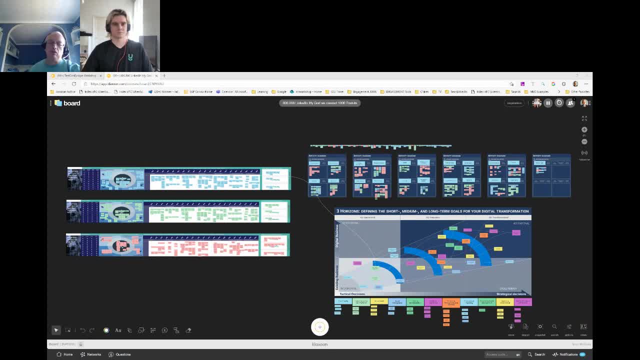 Then of course you need to travel there. So once the workshop is finished, designed that's like one day for the preparation and for the follow up, So during the documentation you usually can say at least two or three days, meaning something like 16 to 20. 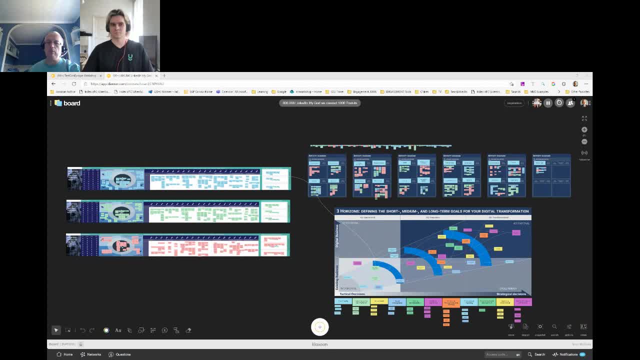 hours for actually writing out the full documentation of the workshop. Thank you, Let's go to the next question: What tools are better to use for building a billboard? Yeah, so the way I do those billboards, I create all of them in PowerPoint, and that's also the templates they share in LinkedIn. 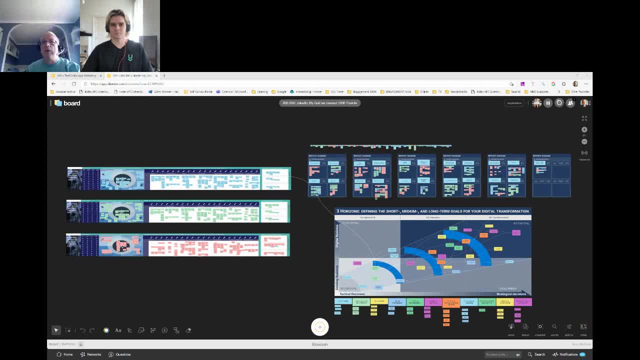 And the reason. there are two reasons for that. First of all, I wanted to kind of enable as many people as possible and not force them to. all you need to go and buy an Adobe Photoshop or an Adobe Illustrator or any tool. So this is, and just like one billion people using it. 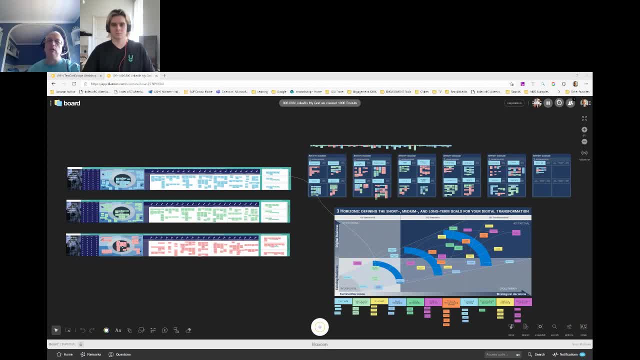 But the second, maybe more important point is you might be very skilled at creating those templates, But before I have a workshop I traditionally will always send it to the customer, because it can always be small wordings. Let's say one: one company will talk about sales manager and the other will call. 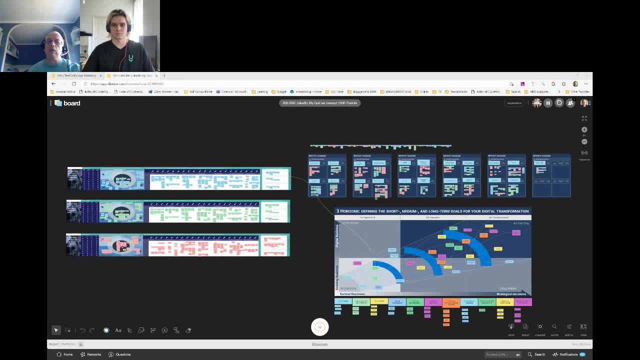 about sales representative and really eager to remove all, let's say, misunderstandings in the workshops. and it can be small things And if you're doing it in PowerPoint, I just can send it to the customer. They can look over it, They can change the wordings. 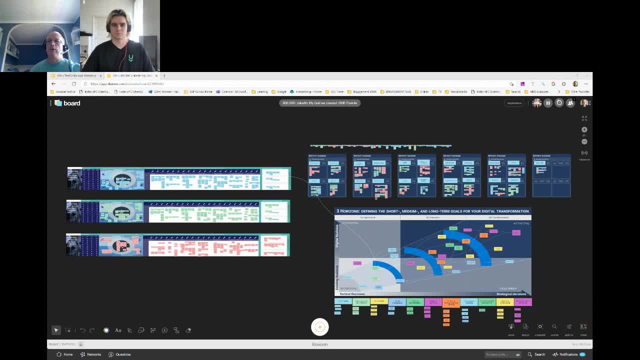 Maybe they don't like a picture or they want to change some colors, But I'm really giving them the full responsibility or the possibility to change. If they say: everything's fine, fine, And I'll just take that PowerPoint and import it into Flexzone. 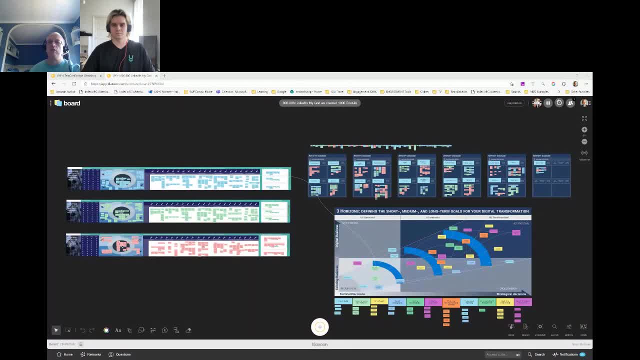 You also can find some videos how to do it. It's not straightforward. You need to select the PowerPoint, the complete graphic, and import it into into paint, cut it into different parts and then import it into Flexzone. But all of those visuals you're ever going to see that I share are all created in PowerPoint.